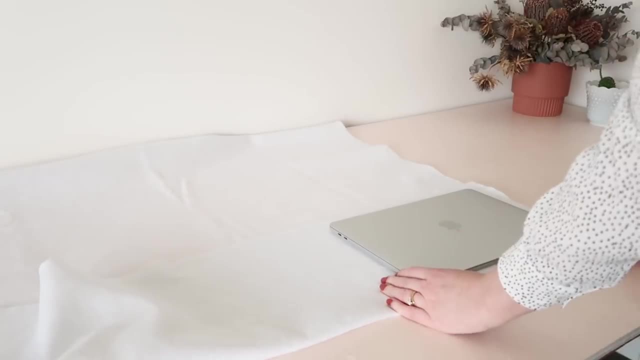 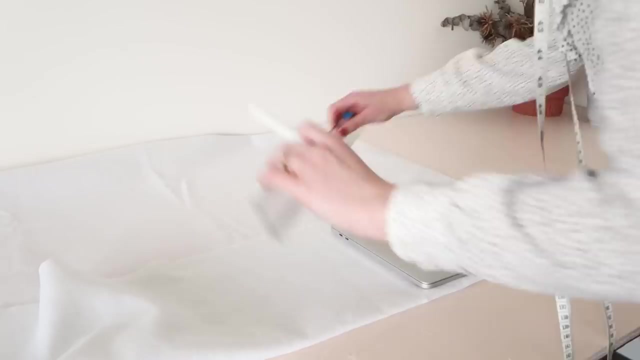 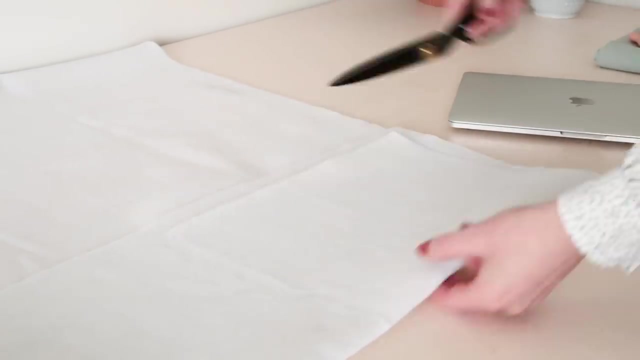 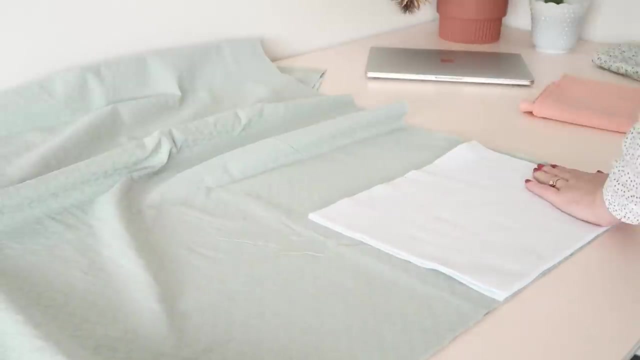 Place your laptop onto your wadding- My laptop is a 13-inch MacBook for reference- and cut out two pieces that are approximately 2.5 centimetres or an inch bigger than the laptop itself. Then cut out two pieces of your main fabric that are the same size, and then two. 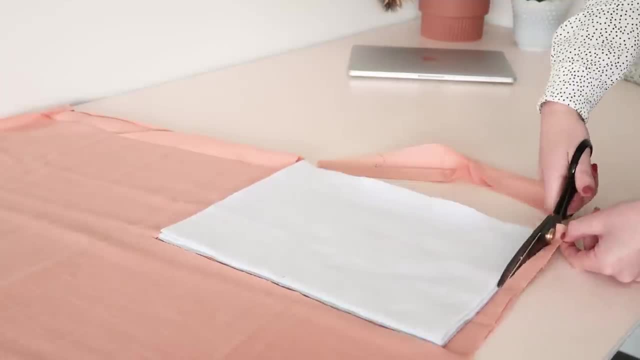 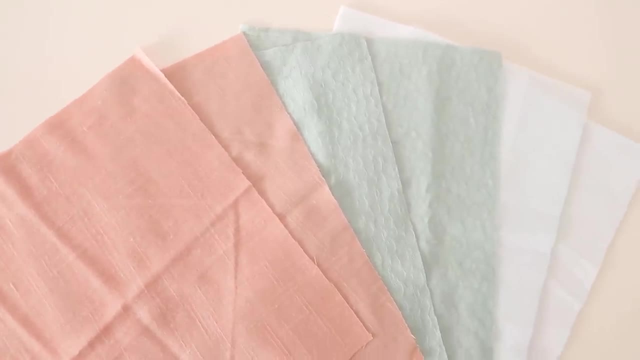 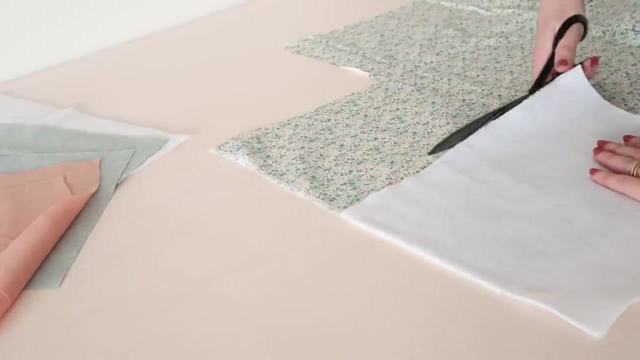 of the lining fabric as well, So you should now have two rectangles of each material that are the same size. We're also going to be making a pocket on the front And for this cut out a rectangle that is the same width as the other rectangles we just cut out by. 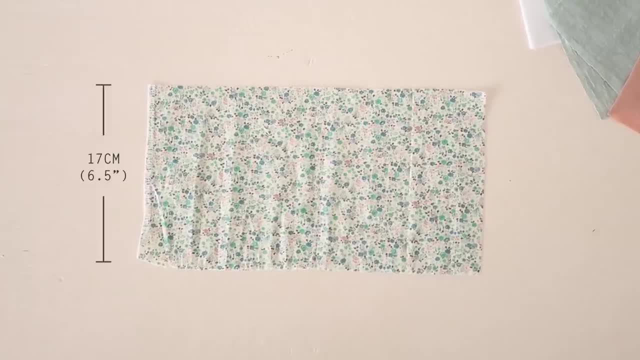 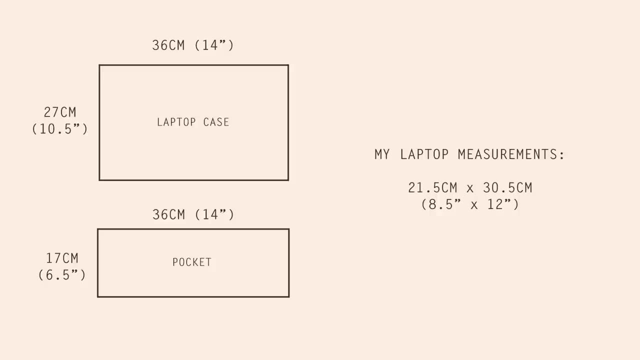 however big you'd like your pocket to be, I made mine 17 centimetres, or 6 and a half inches, So for my laptop case. here are the dimensions I cut out. Start by taking the pocket rectangle and fold and press the top edge in by about one centimetre. 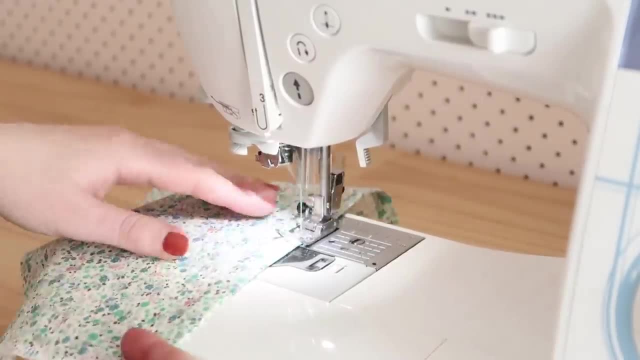 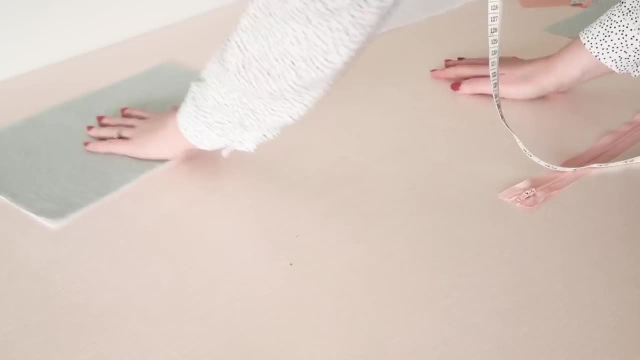 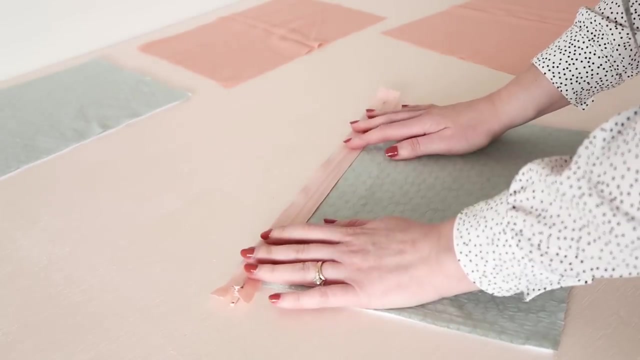 or half an inch twice, Then stitch the folded edge in place. Next, place the main fabric onto the felt with the right side of the fabric facing up and with right sides together. place the zip along the top edge of the main fabric and then place. 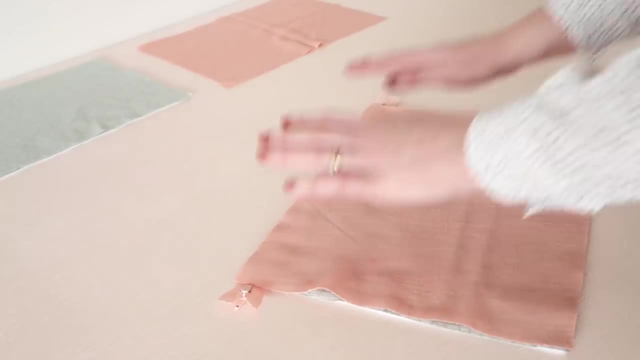 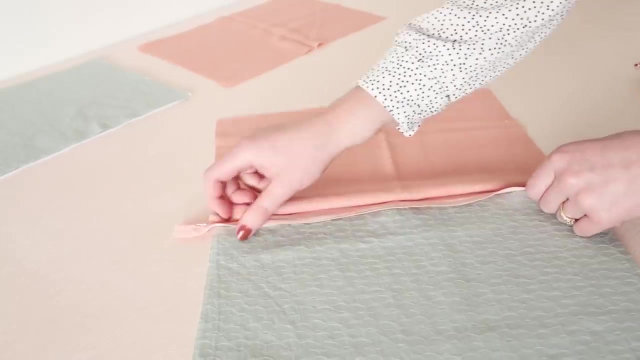 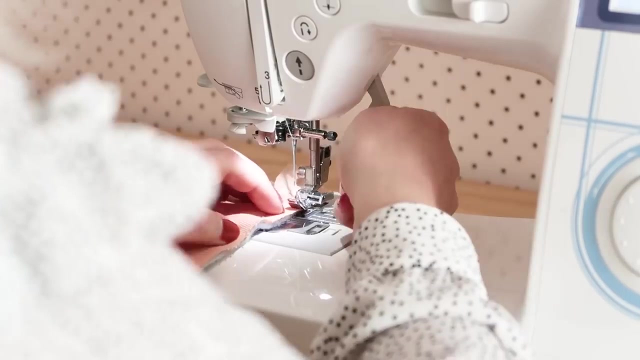 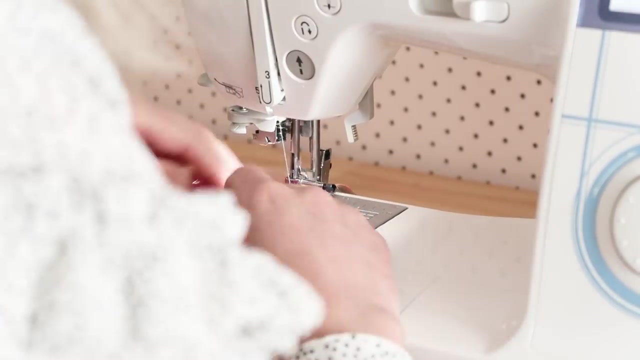 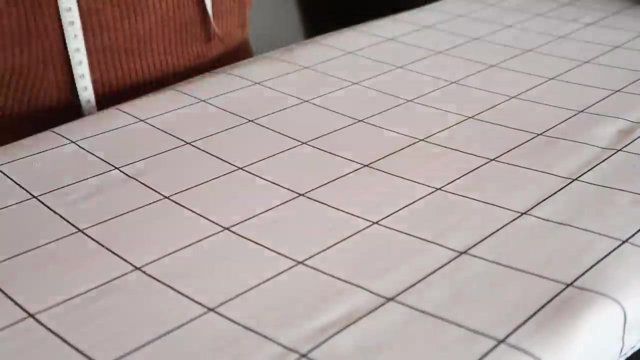 the lining fabric on top, making sure that the right sides of the main and lining fabrics are facing. pin all of the layers together, sandwiching the zip in between the layers of fabric. then stitch the zip and the fabrics together. once stitched, half of the zip should be nicely enclosed in between the layers of. 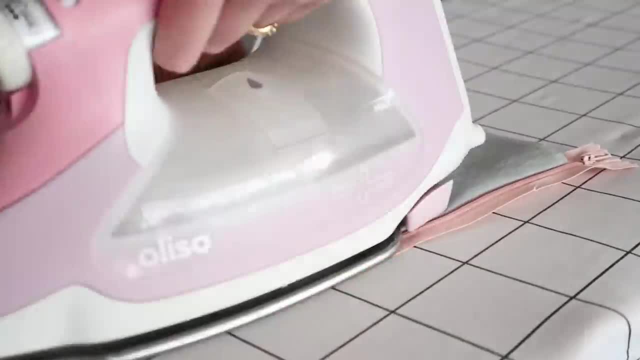 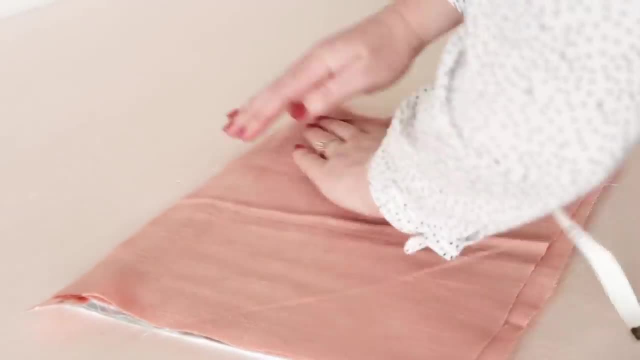 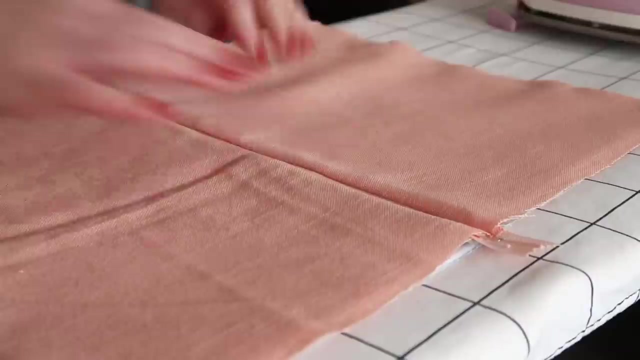 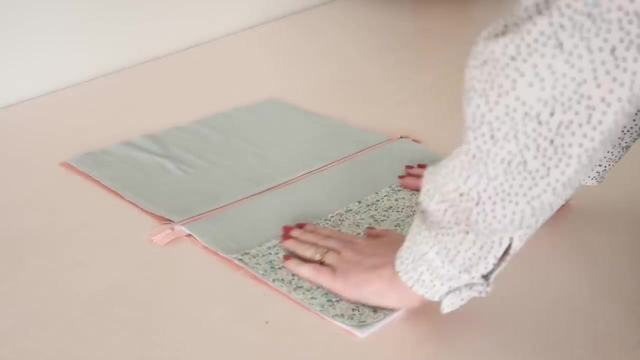 fabric. then simply repeat the stitches for the other side of the zip and the remaining rectangles of fabric and you should now have something that looks like this: next place the pocket piece we made earlier onto one of the main fabric rectangles, and then open the zip slightly and fold the other main fabric. 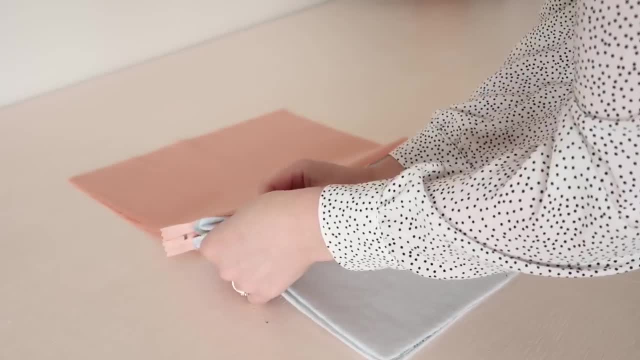 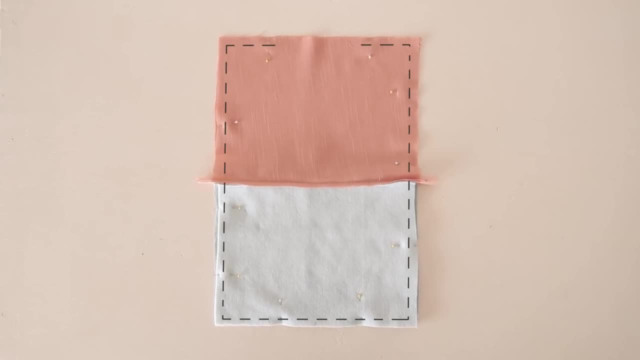 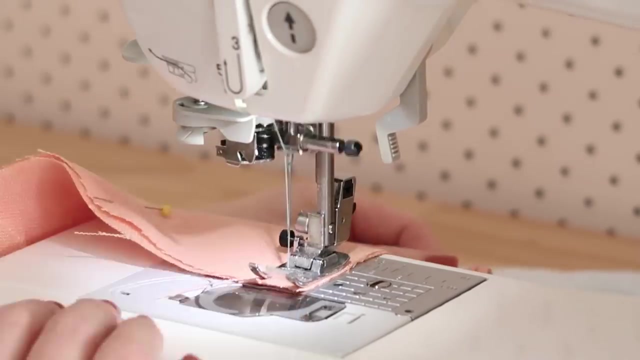 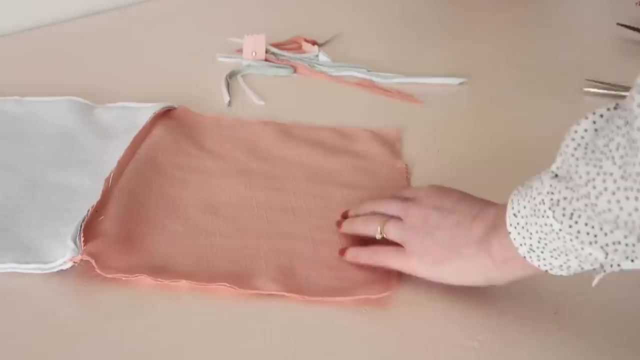 rectangle with the felt layer on top, also flipping the linings together. stitch the layers together, leaving an opening at the top of the lining like this. trim away the excess fabric and then, using the opening in the lining, turn the laptop case right side out. use something like a knitting needle to poke out the corners. 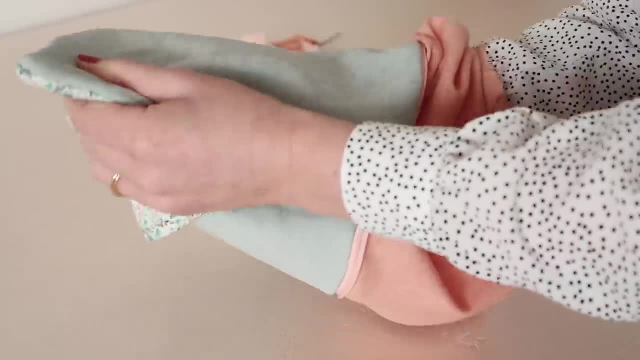 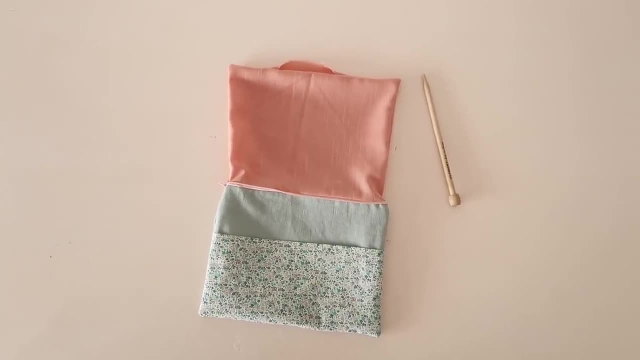 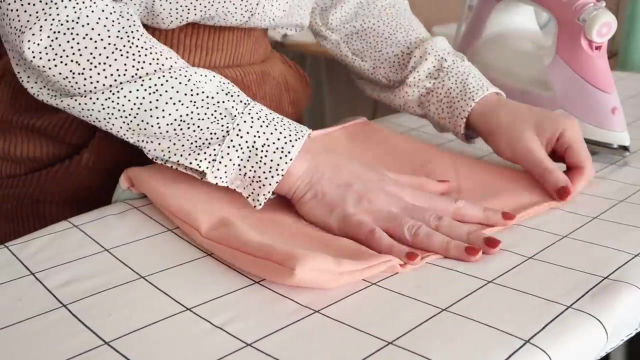 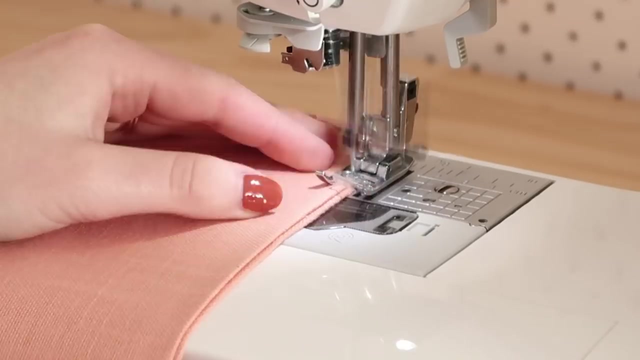 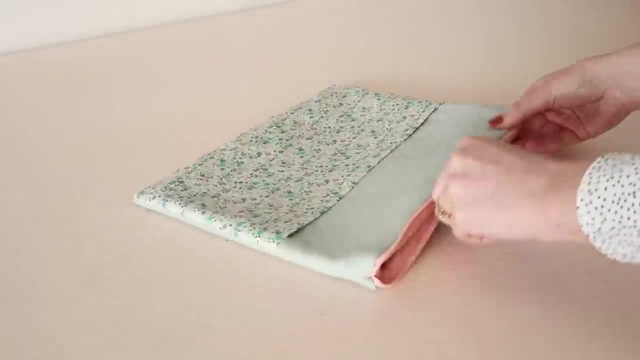 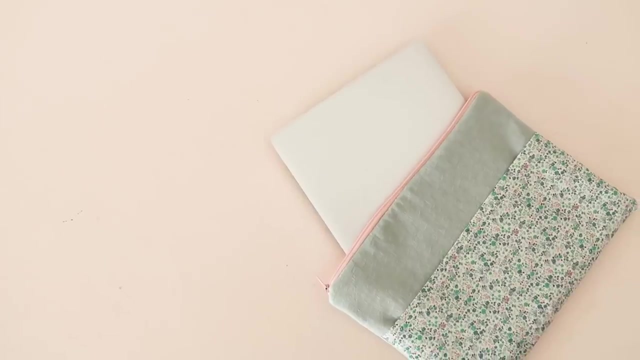 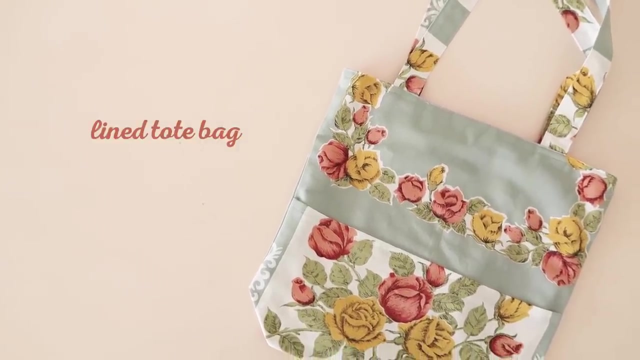 foreign. until you have something that looks like this: give the case a good press and then stitch along the top edge of the lining like this. then simply tuck the lining inside and your laptop case is complete. next, let me show you how to make this fully lined tote bag. 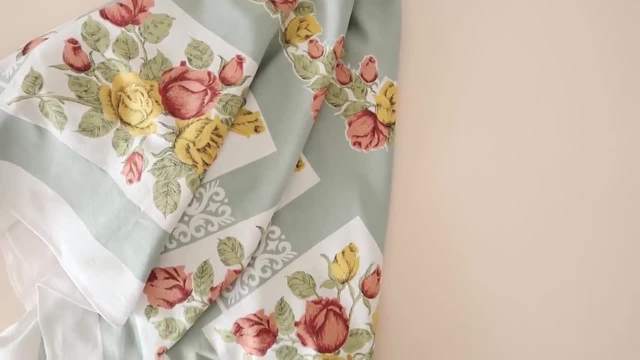 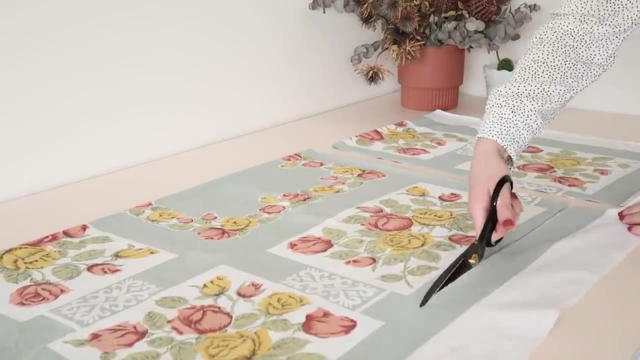 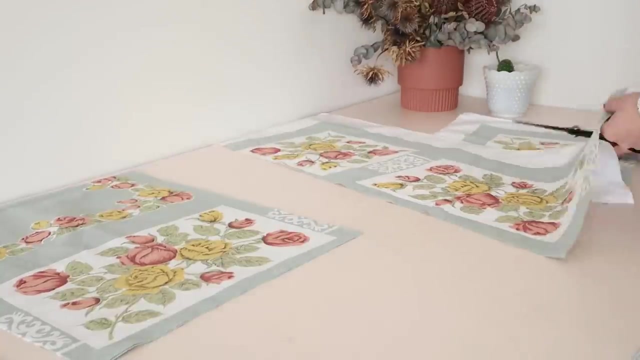 for this project I'm using a recycled tablecloth, but any mid to heavyweight fabric will work fine. start by cutting out two rectangles that are approximately 45 centimeters or 8 inches, by 50 centimeters or 20 inches, and a smaller rectangle that's approximately 45 centimeters or 18. 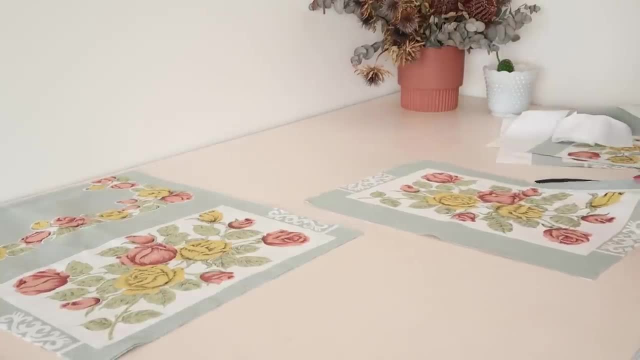 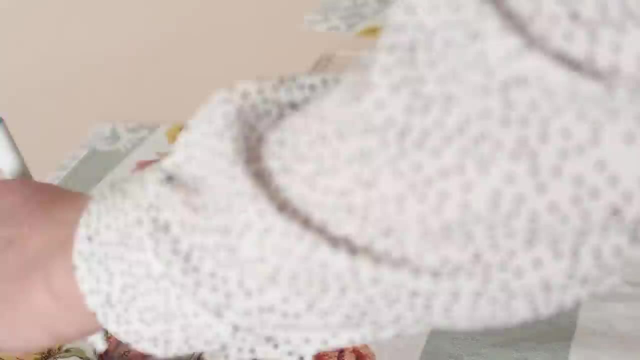 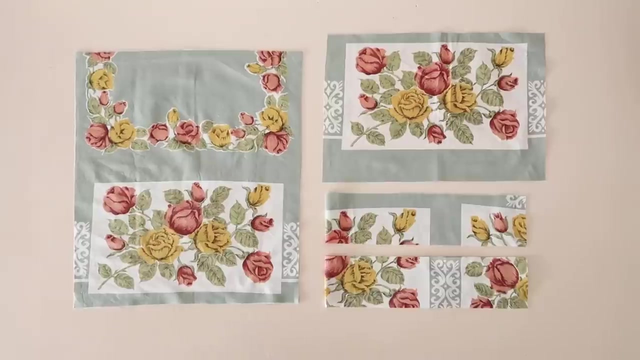 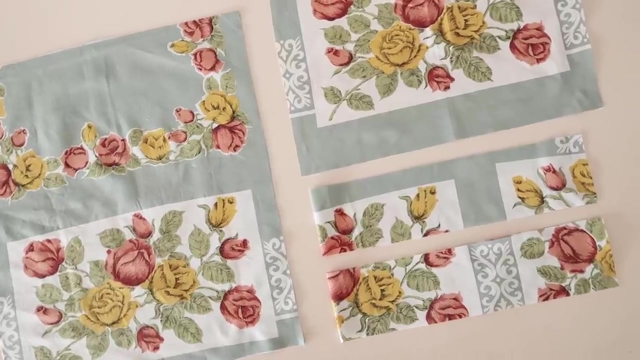 inches by 30 centimeters or 12 inches. then cut out two more rectangles that are approximately 80 centimeters or 31 and a half inches, by 10 centimeters or 4 inches. so you should now have the following pieces: take the longer rectangles and fold and press each long edge in by about one centimeter or 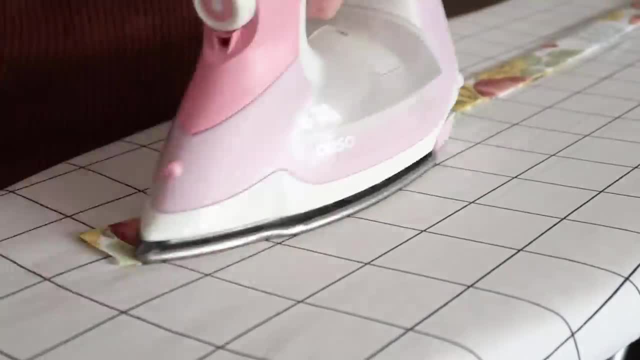 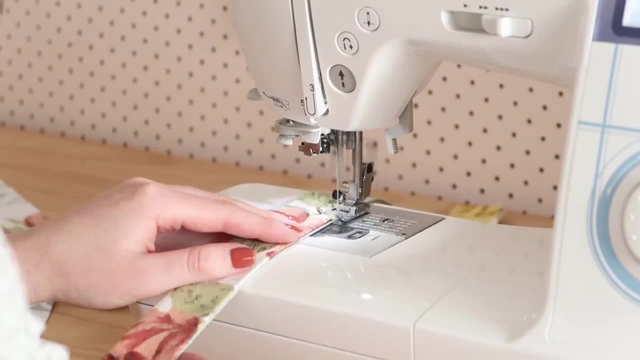 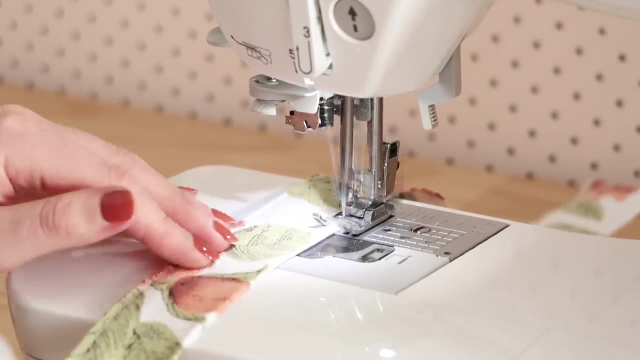 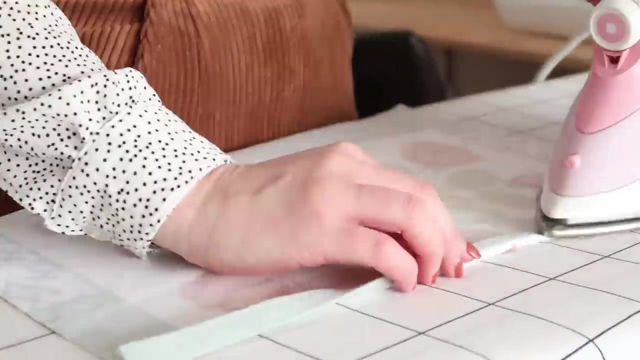 half an inch and then fold and press the rectangle in half. Stitch along both sides of the rectangle. these are going to be the straps of the bag. next, take the smaller rectangle and fold and press the top Edge by about one centimeter or half an inch twice. Then stitch the folded edge in. 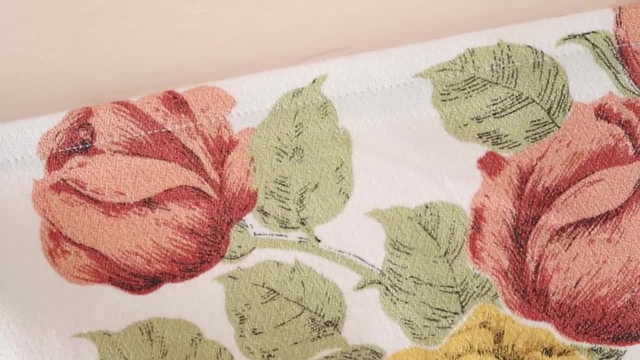 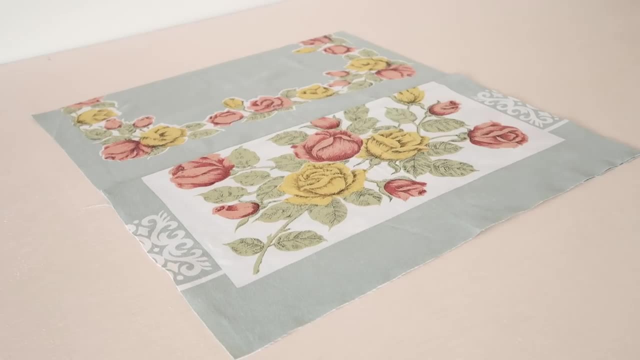 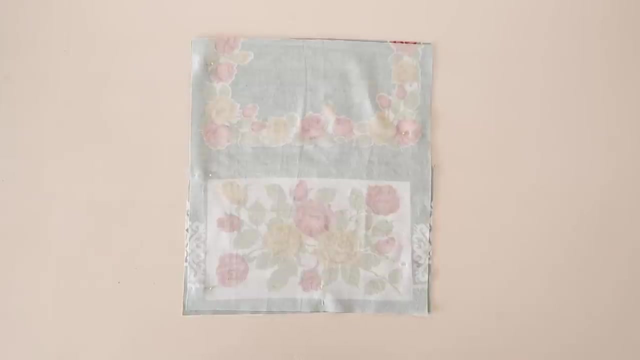 place. This will be a pocket for the front of the bag. Place the pocket onto one of the larger rectangles, lining up the raw edges together, Then, with right sides together, place the other large rectangle on top, sandwiching the pocket in place. Stitch all of the layers together, leaving the top open like this. 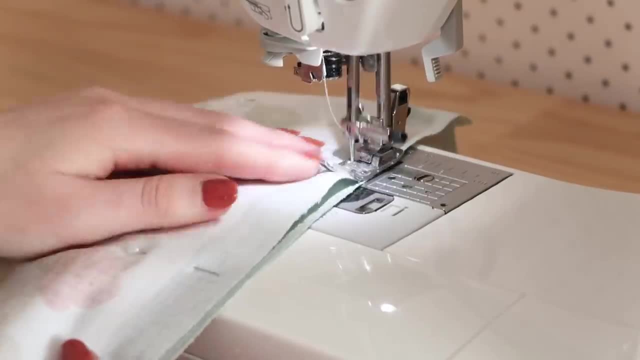 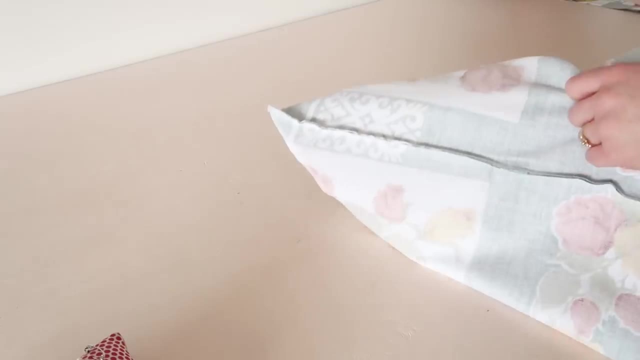 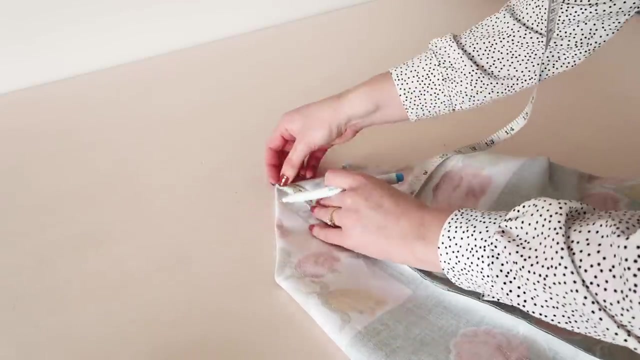 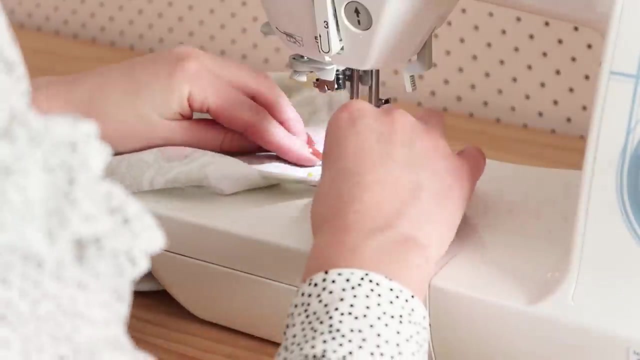 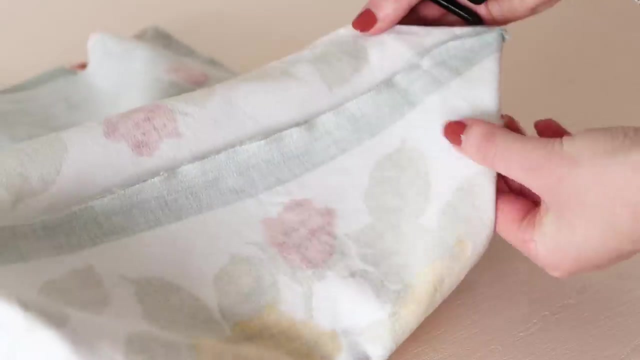 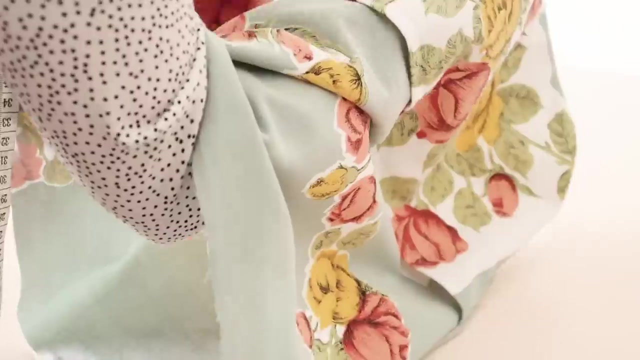 Trim away the excess fabric and then fold the bottom corners into a point and then pin and stitch approximately five centimeters or two inches from the corner point. Trim away the excess fabric at the point and then turn the bag right side out. This step creates a fold at the bottom of the bag, to make it a little bit. 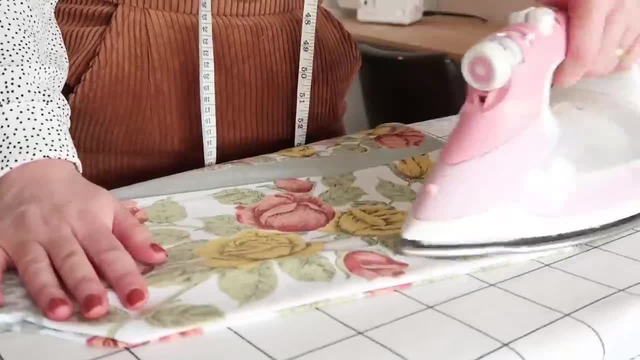 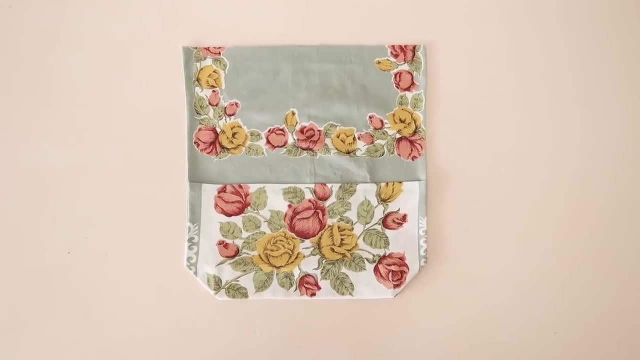 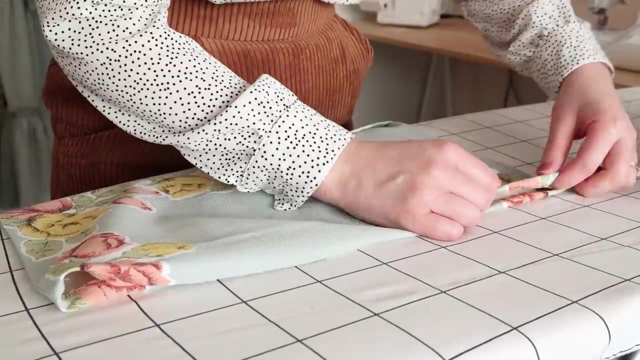 roomier and to be able to carry bulkier items. Give the bag a good press and it should now be looking a little something like this: Trim off the excess fabric, Next fold and press the top edge of the bag in by about one centimetre or half. 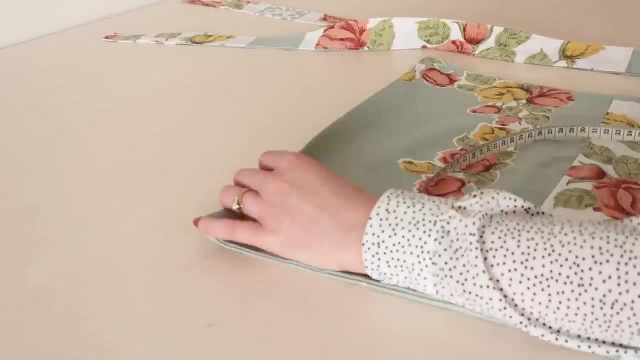 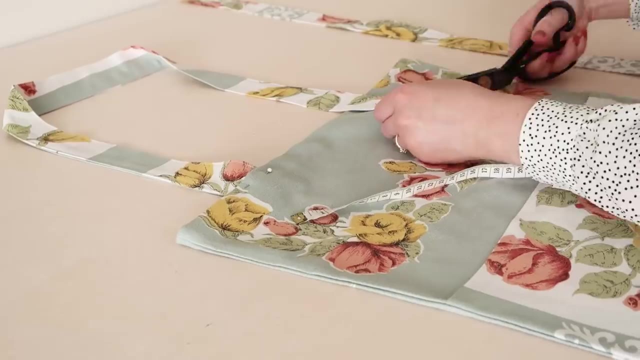 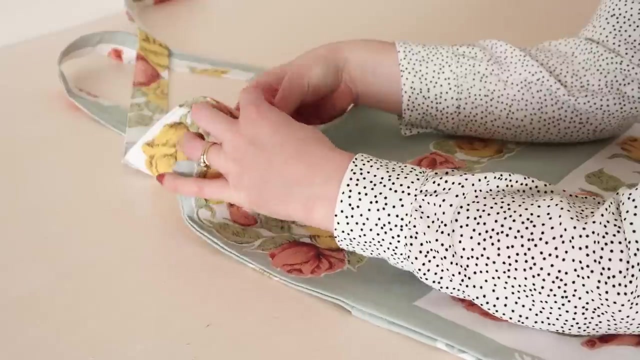 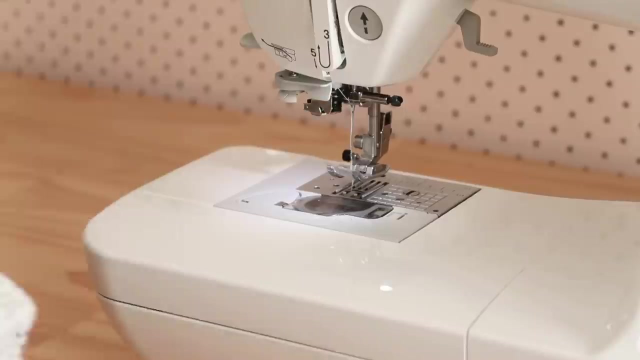 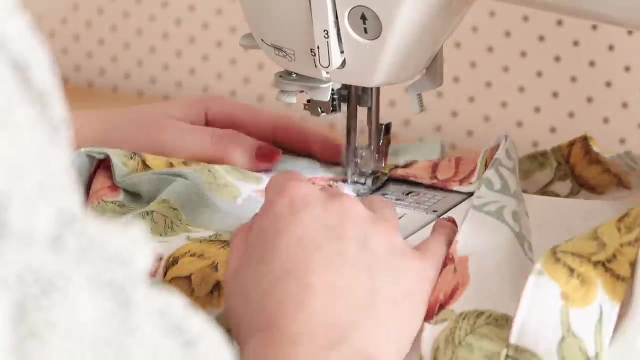 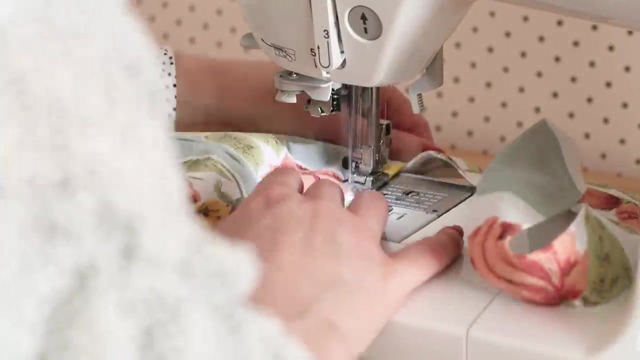 an inch. Then pin the straps into the folded edge, making sure they're positioned the same distance away from the edge of the bag. Stitch the folded edge in place, securing the straps as you sew. Now, at this point you have a fully functioning tote bag. but let me quickly. 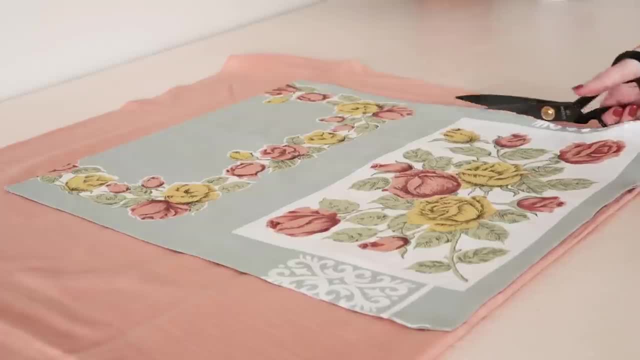 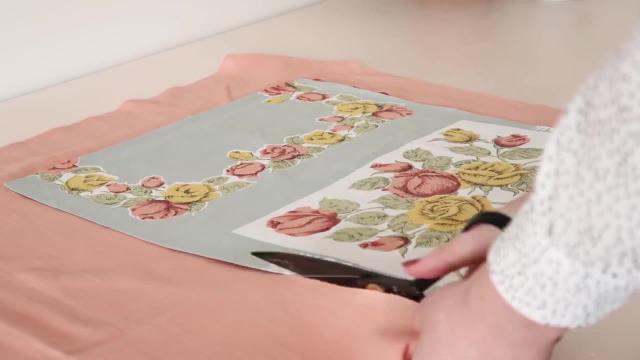 show you how to also add a lining. Start by cutting out two rectangles that are the same size as the bag rectangles in a lining fabric. I'm using a contrasting fabric that is also salvaged from an old tablecloth. I'm also going to be adding 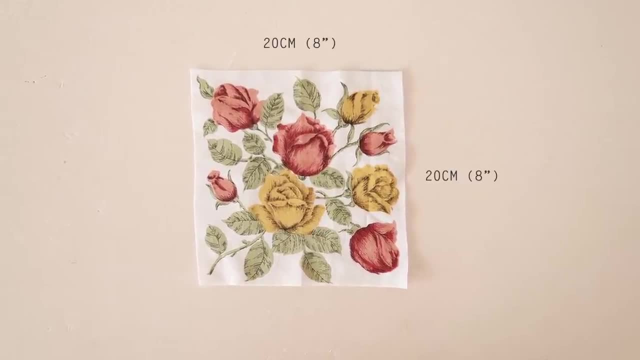 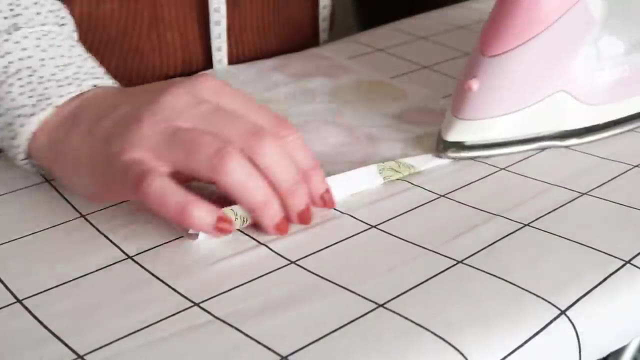 an interior pocket and for this I cut out a 20 by 20 centimetre or an 8 by 8 inch square of fabric. Take the pocket piece and fold and stitch the top edge in by about one centimetre or half an inch twice. 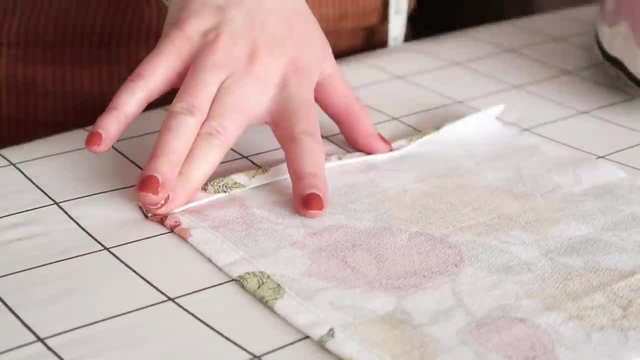 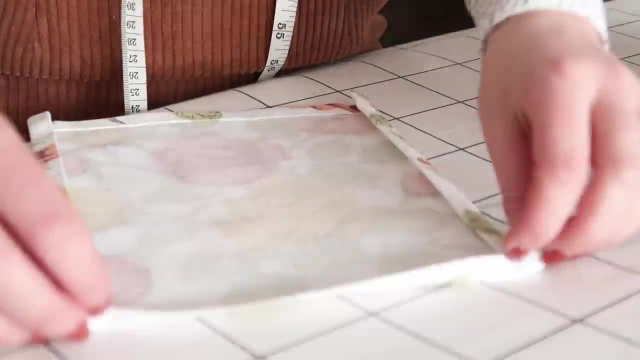 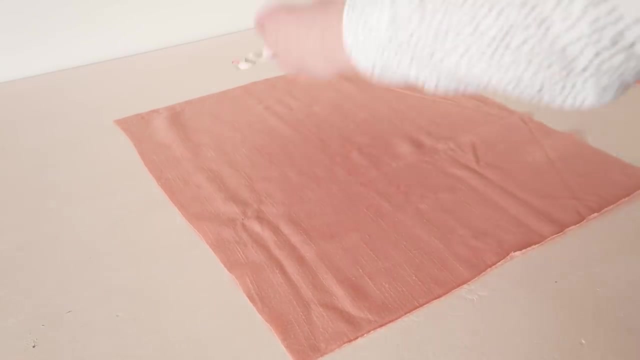 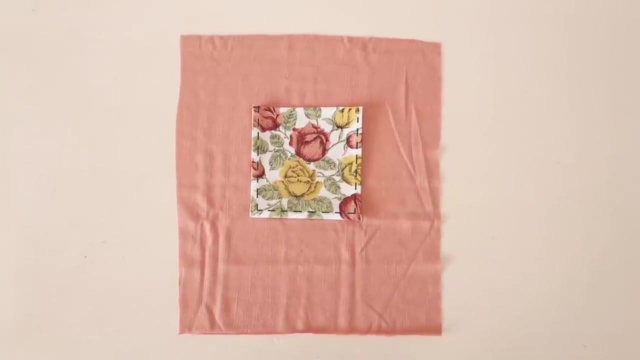 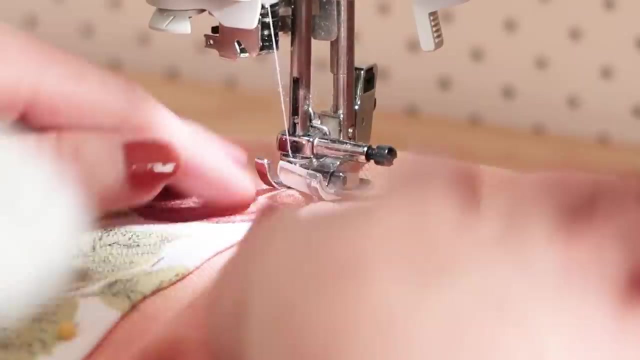 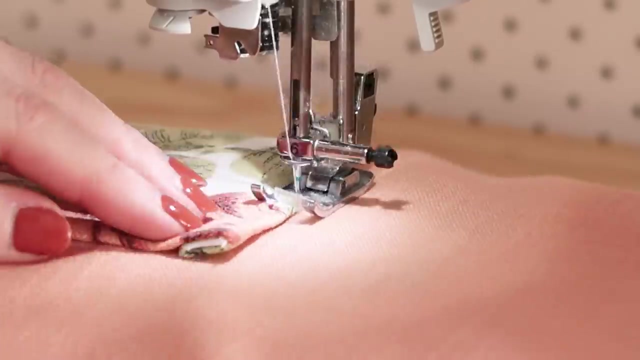 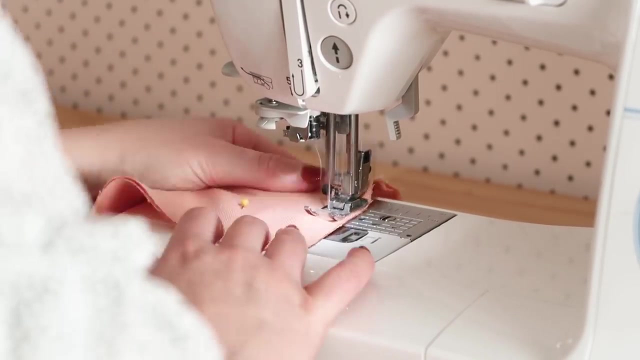 Then do the same for the remaining edges, but don't stitch them just yet. Take one of the lining rectangles and place the pocket onto it. Then stitch the pocket in place along three of the edges like this. Then simply stitch up the lining as we did for the main bag. 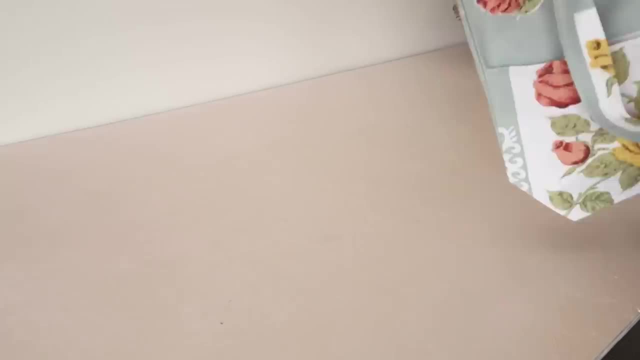 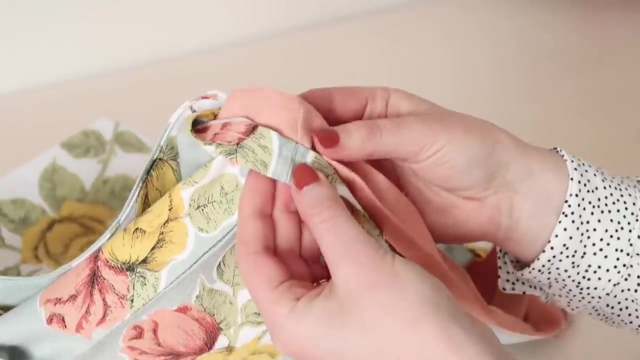 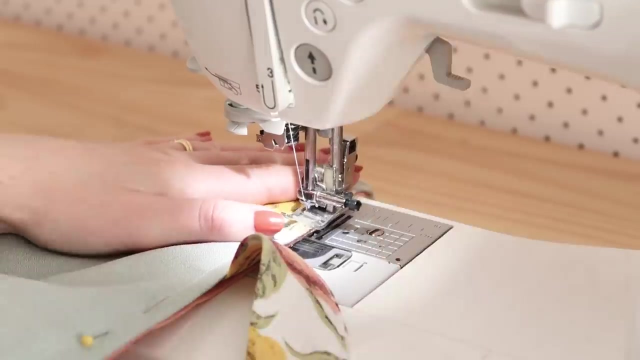 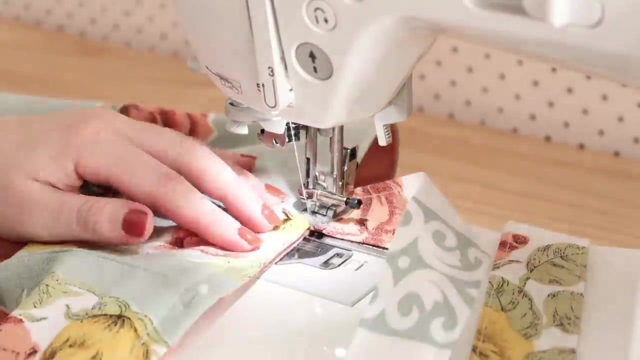 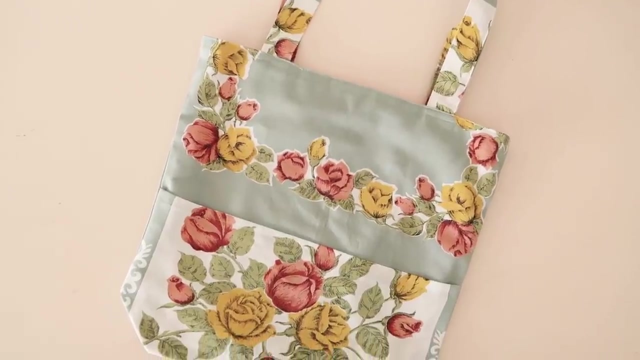 Now with wrong sides together, place the lining inside the bag and then pin the lining to the bag along the top edge, matching the side seams together. Top stitch along the top edge of the bag, stitching the lining in place as you sew, And your lovely fully lined tote bag is complete. 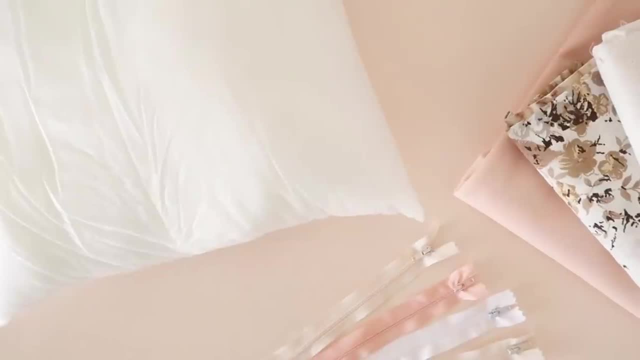 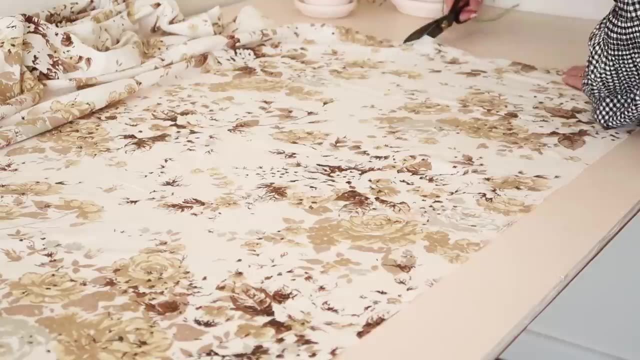 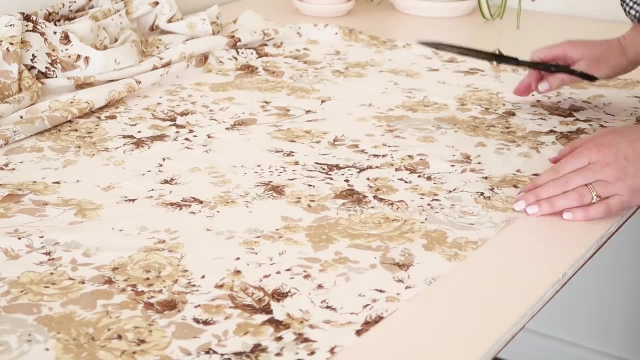 Next, let me show you how to make a ruffled cushion cover For this project. you'll need a 40cm or 15.5 inch zip and about 3 quarters of a metre or 3 quarters of a yard of fabric. Cut out one 40x40cm or 15.5x15.5 inch square, one 30x40cm or 12x15.5 inch rectangle, and 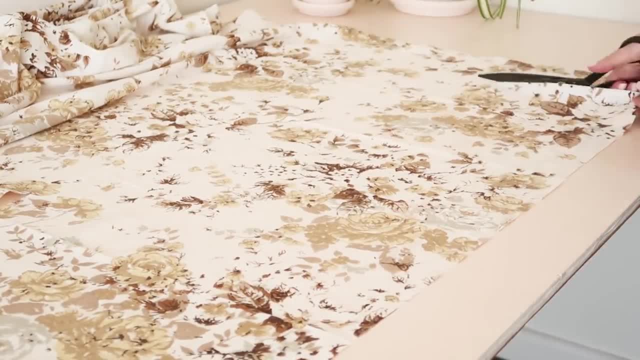 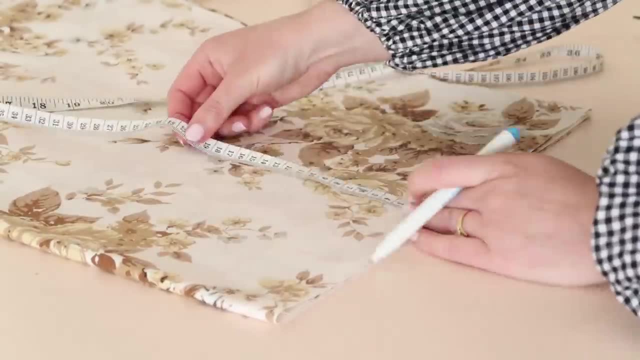 one 15x40cm or 6x15.5 inch rectangle For the ruffle. also cut out one 15cmx4m or 6x4 inch rectangle. It's absolutely fine to cut out the ruffle in multiple pieces and then stitch them together. 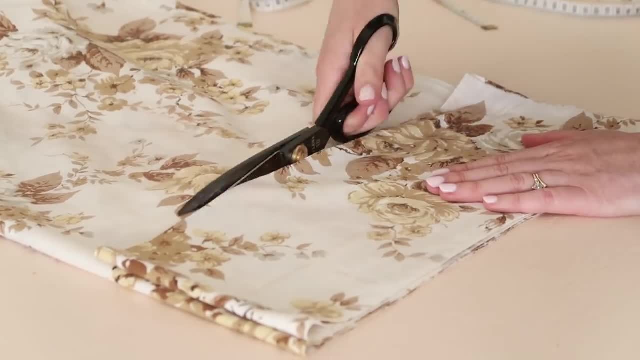 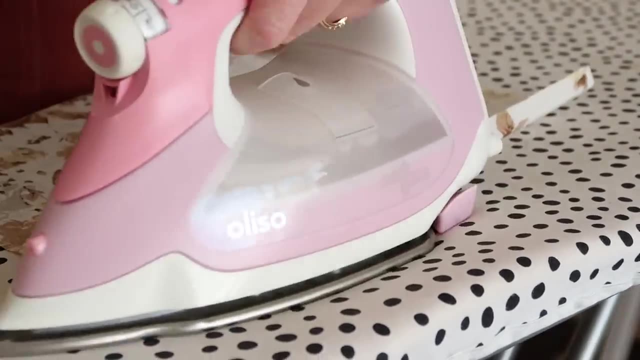 to make the 4m length of fabric. So all up, you should have the following pieces: Take the larger rectangle and press one of the longer edges in by about 1cm or half an inch. Then, with the right side of the zip and the fabric facing forward, cut out the ruffle. 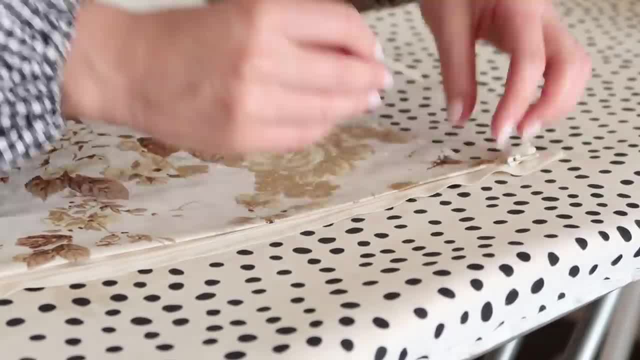 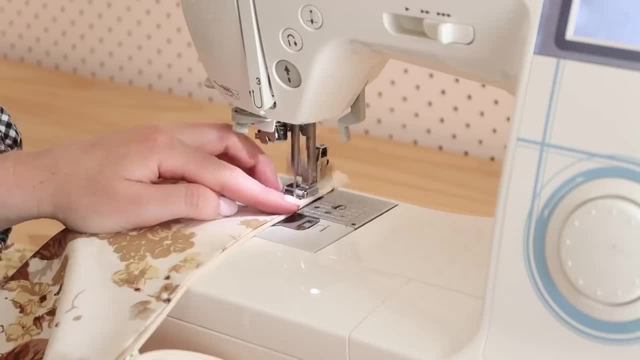 Then, with the right side of the zip and the fabric facing forward, cut out the ruffle. Then, with the right side of the zip and the fabric facing up, place the folded edge up against the teeth of the zip, Pin the fabric in place, making sure that the zip can still open up properly. 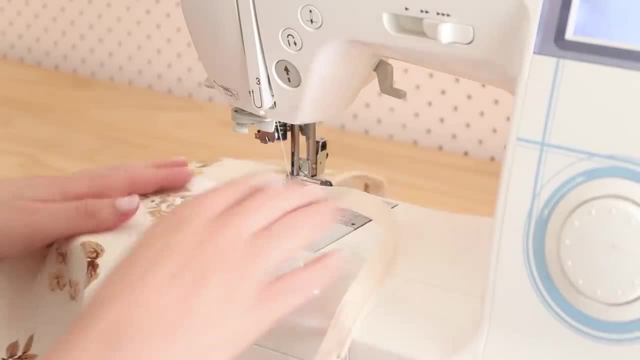 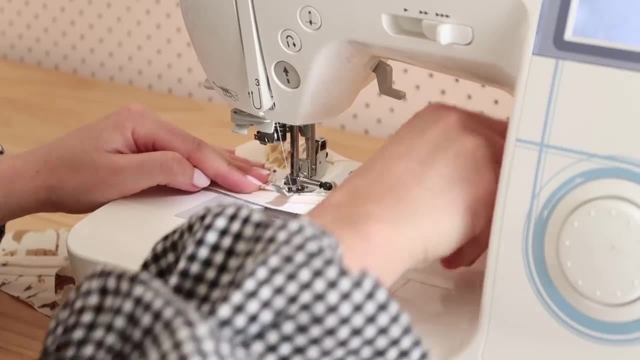 Next stitch the zip in place by lining your zipper foot along the teeth of the zip. When you get to the zip slider, simply place your needle down into your fabric, turn your fabric slightly and zip the zipper shut to get it out of the way so that you can continue. 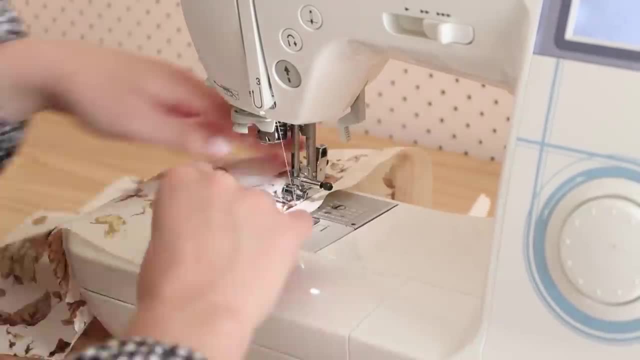 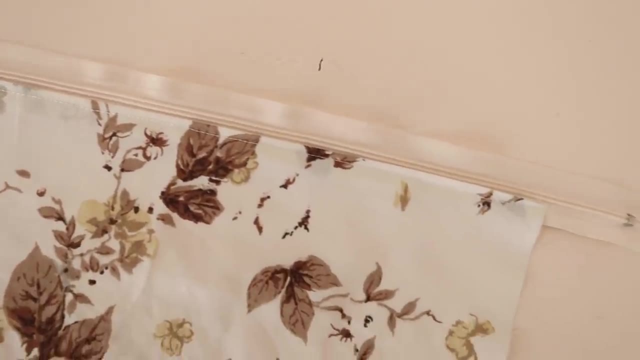 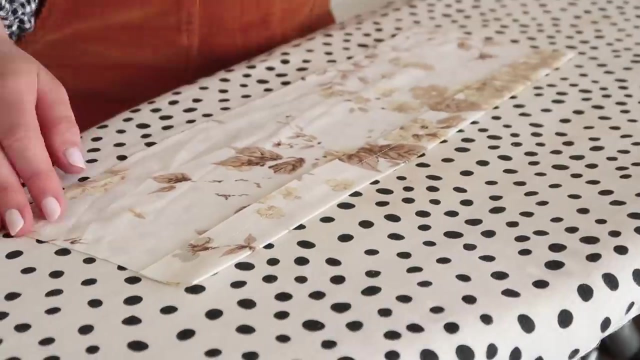 sewing easily And your zip should now be nicely attached to your fabric like this. Next, take the smaller rectangle and this time press one of the longer edges in by about 2 and a half cm or one inch. Then, with the right side of the zip and the fabric facing down, place the zip onto the 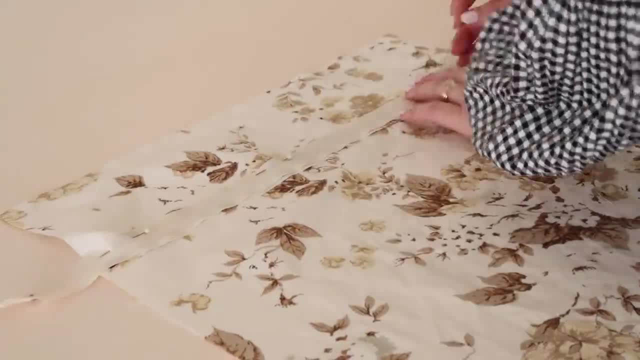 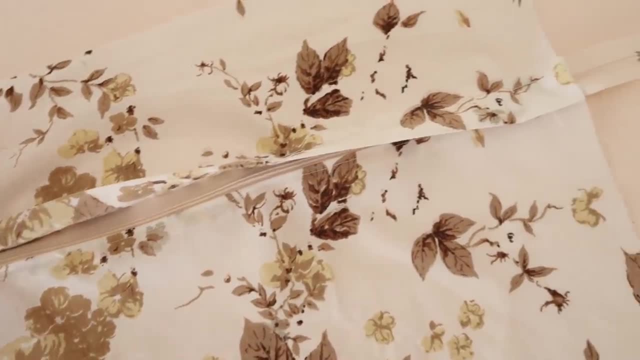 folded fabric Pin in place, making sure the folded edge covers up the zip like this. Then place the zip onto the folded fabric Pin in place, making sure the folded edge covers up the zip like this. Then place the zip onto the folded fabric. 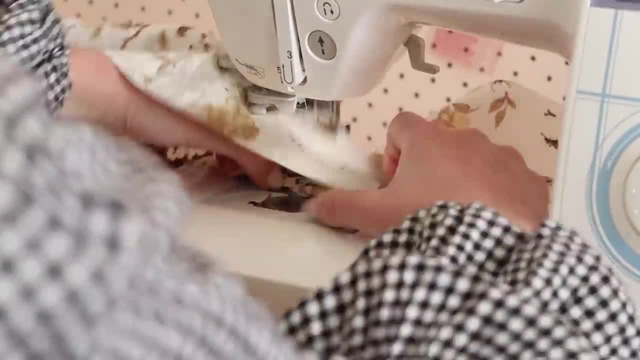 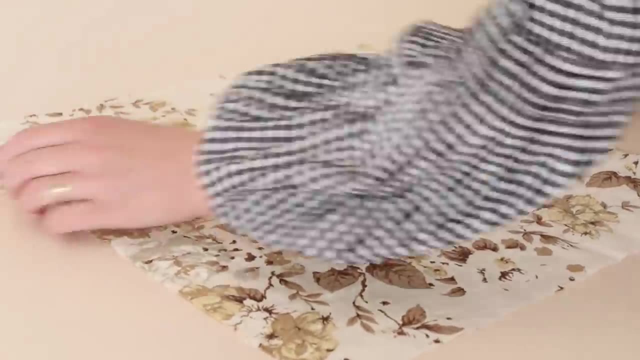 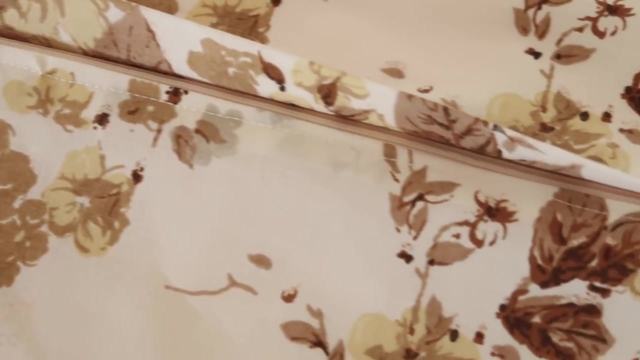 Then stitch the zip in place again, lining up the zipper foot along the teeth of the zip, And you should now have another 40x40cm or 15 and a half by 15 and a half inch square of fabric with a nicely covered up zip in it like this: 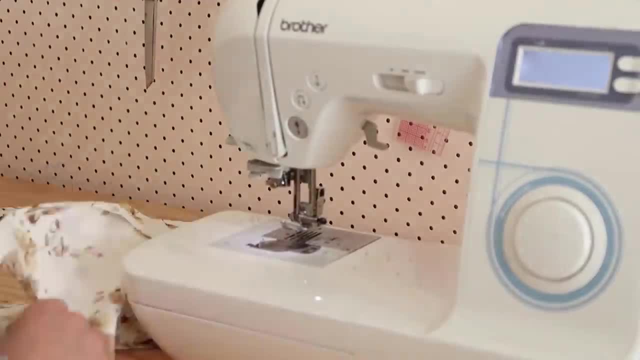 Now to make the ruffle. If you weren't able to get a full 4 metre or 4 yard long piece of fabric for the ruffle, start by stitching together your multiple lengths to get a complete 4 metre piece. Then stitch the zipper in place again, lining up the zipper foot along the teeth of the 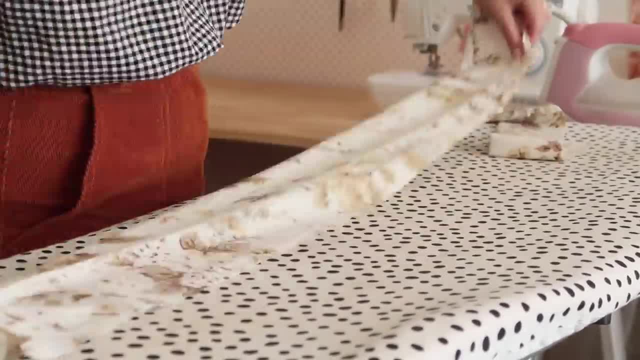 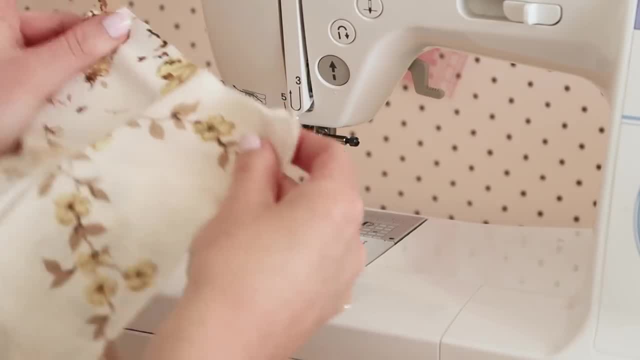 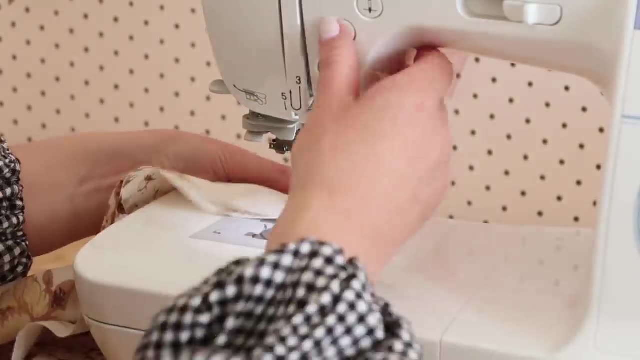 zip. Then, with rung sides together, fold and press your length of fabric in half. Then fold your length of fabric into a loop and stitch the two shorter raw ends together. Change the stitch length of your machine to the longest possible setting and sew two rows. 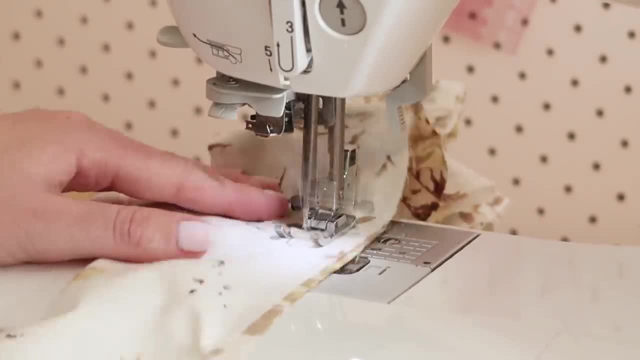 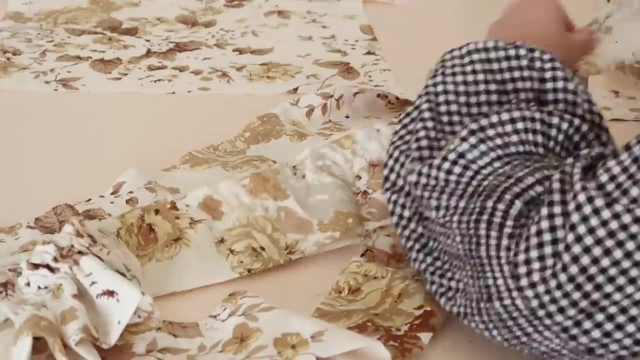 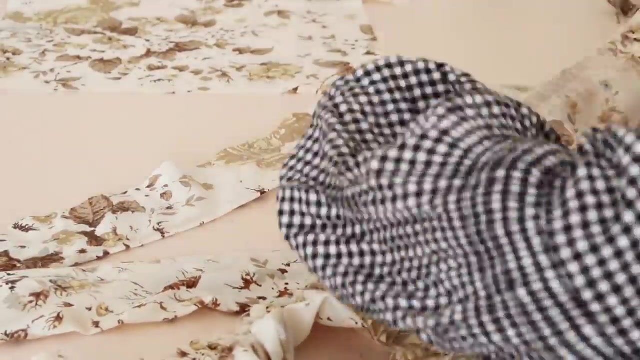 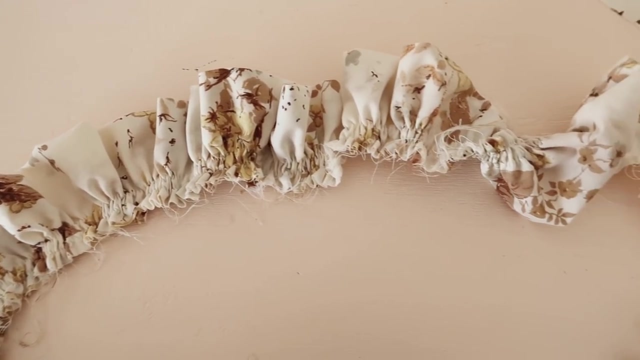 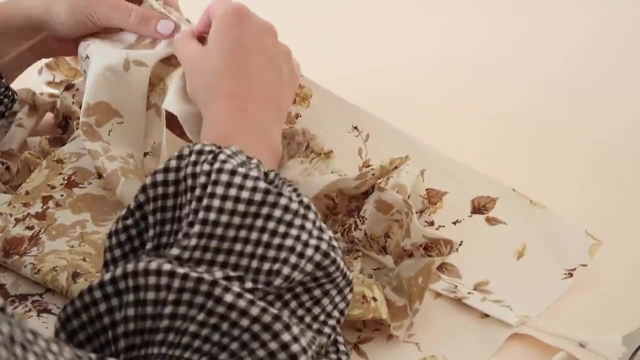 of gathering stitches along the raw edge of your folded fabric, And that's it. Then gather the fabric by gently pulling on the threads until your fabric loop measures the same as the outside edge of the cushion. squares With right sides together. sandwich the ruffle between the two fabric squares by lining up. 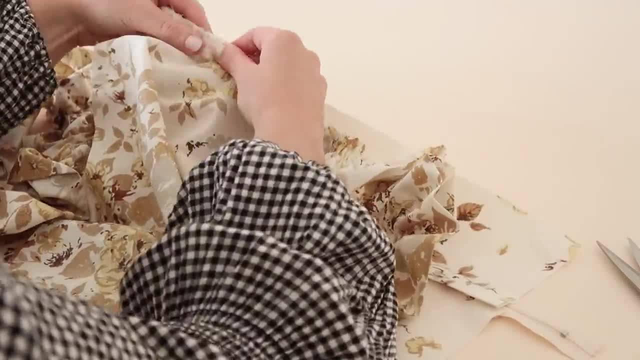 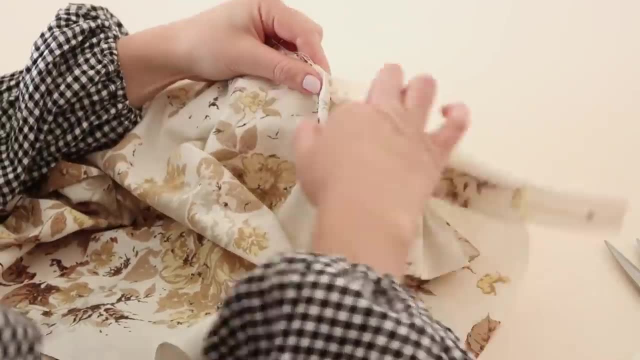 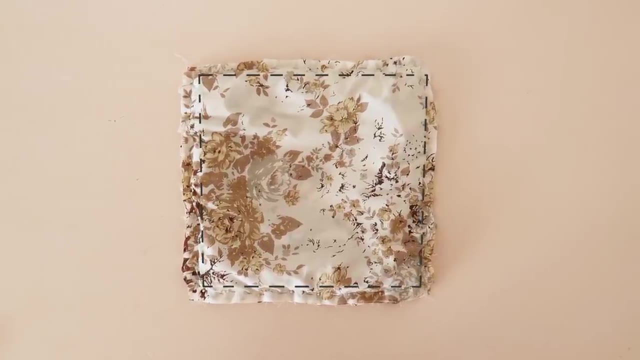 the raw edges and pinning the three layers of fabric together. Then stitch the ruffle around the entire edge of your ruffle to make up for the rough edges that you have seen. Next, stitch around the entire edge like this, making sure your zip is opened slightly to. 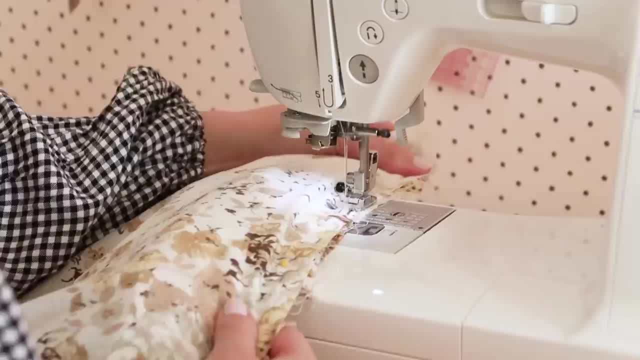 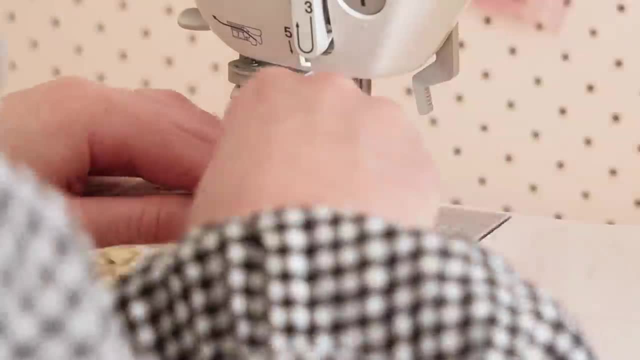 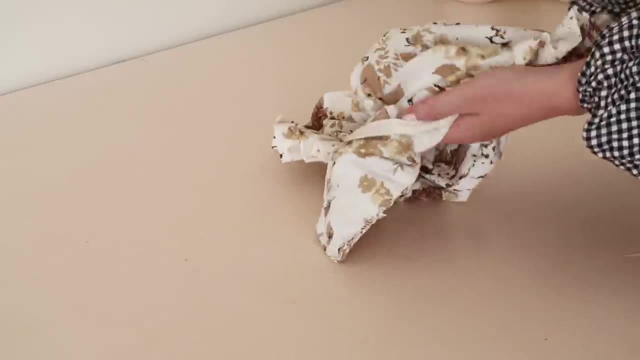 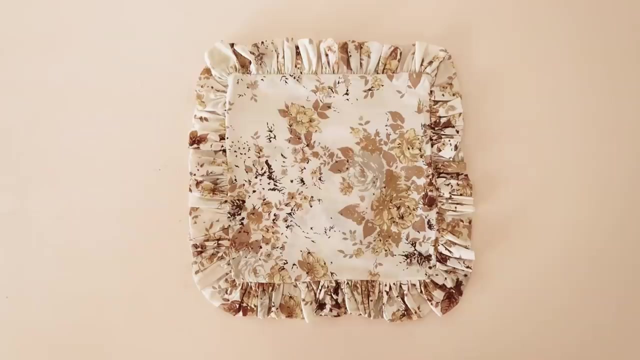 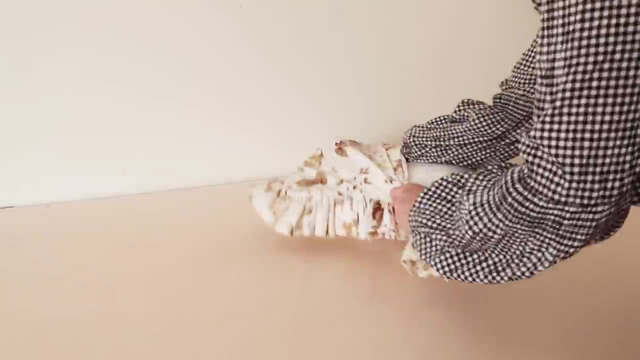 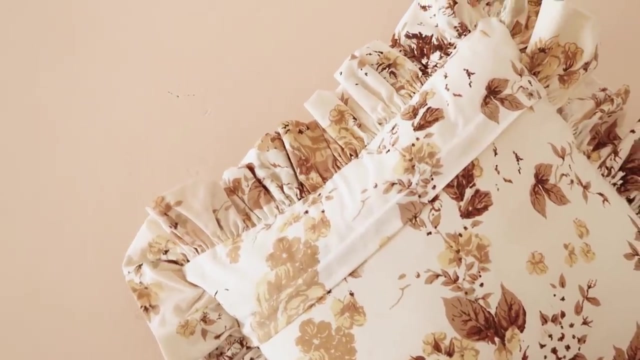 be able to turn your cushion cover right side out. once it's done, Now to fold in the ruffle. Next stitch around the same edge all the way around the ruffle and your lovely ruffled cushion cover is complete. simply squeeze your cushion insert into the zipper opening and you now have yourself an adorable ruffled 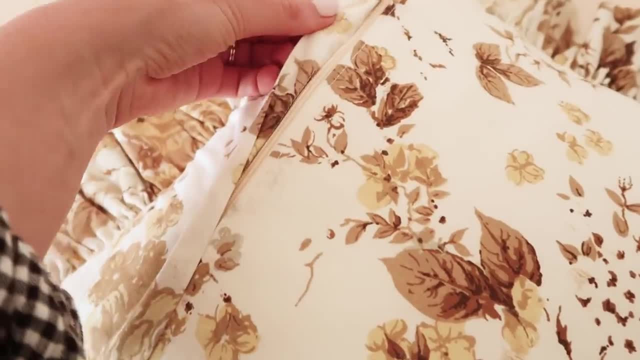 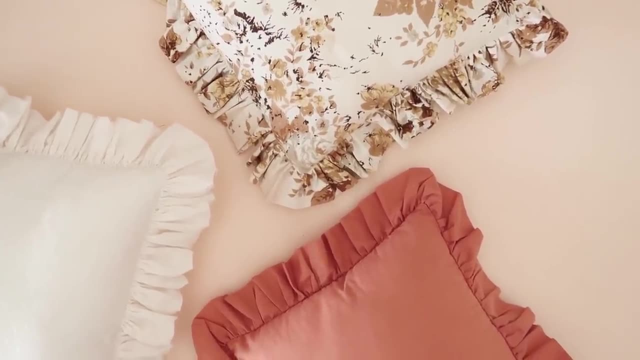 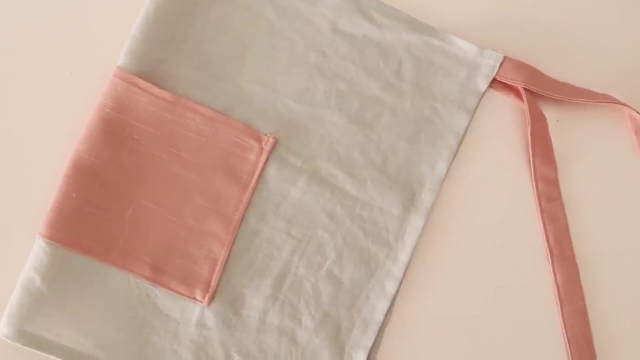 cushion with a nicely hidden zipper opening in the back. lastly, let me show you how to make an adorable waist apron. for this project, you will need a main and contrasting fabric. start by cutting out a 75 by 50 centimeter, or 29, and a. 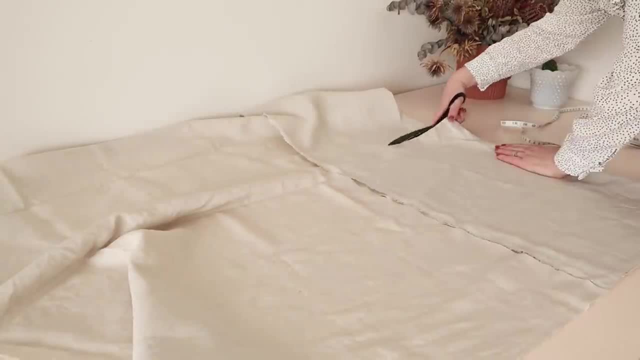 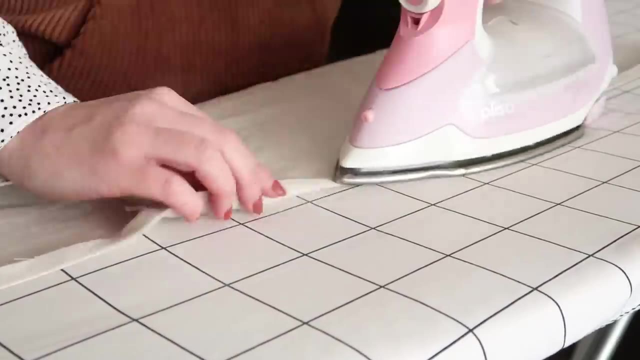 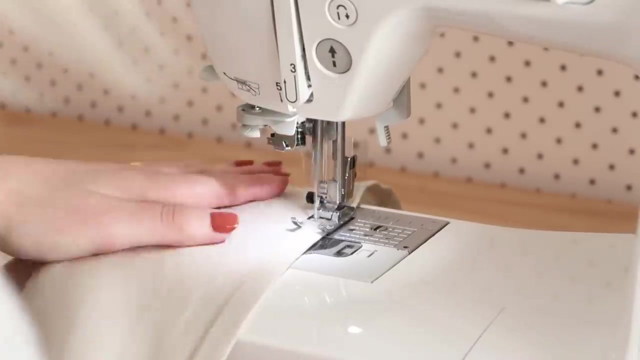 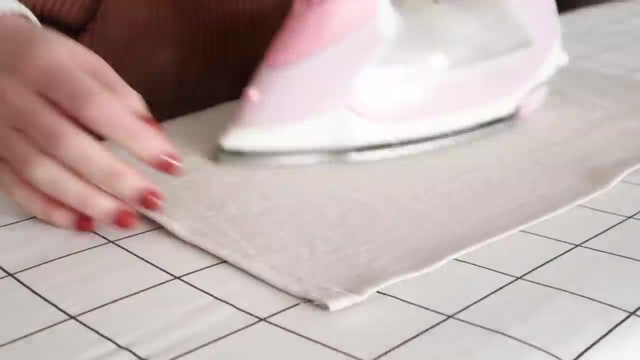 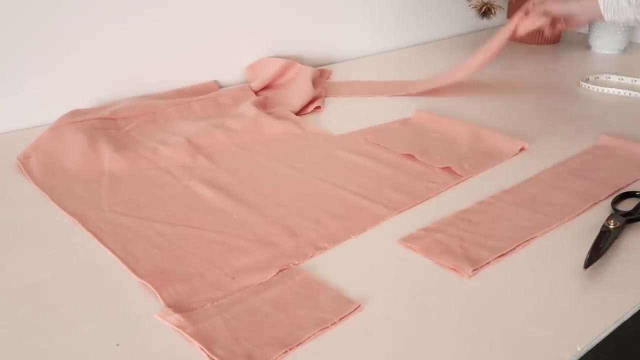 half by 20 inch rectangle in your main fabric. then fold and press each edge in by about one centimeter or half an inch twice stitch all four folded edges in place and then give them a good press. next cut to 100 by 10 centimeter or 40 by 4 inch rectangles and 122 by 42. 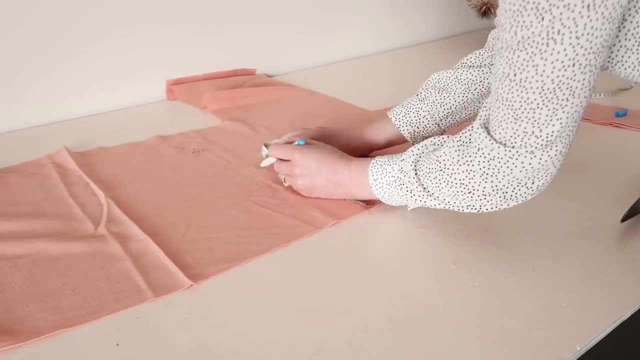 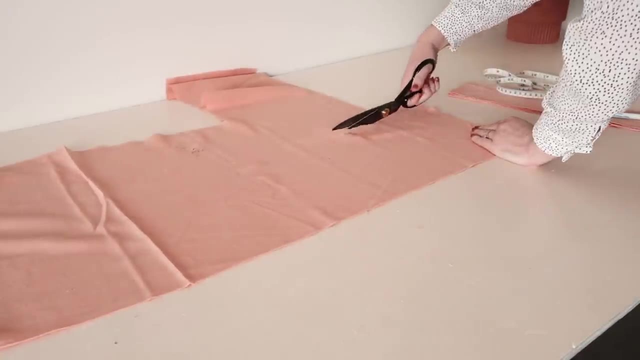 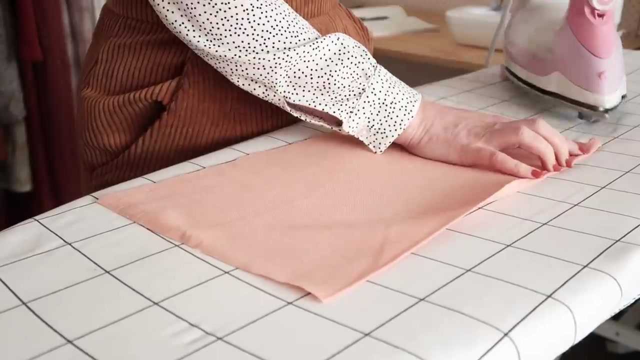 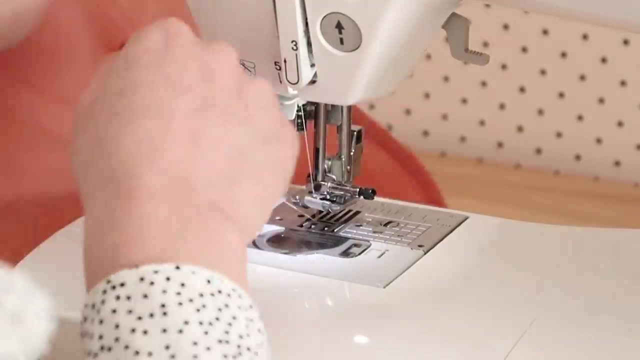 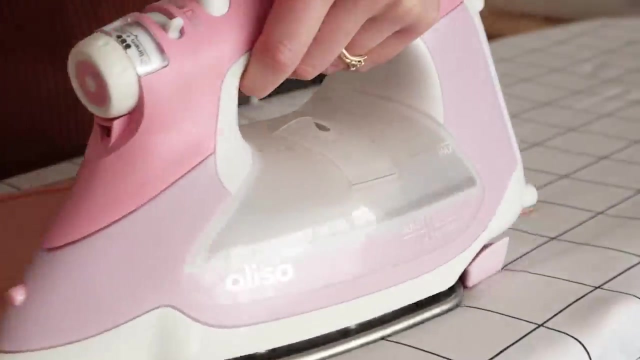 centimeters. take the shorter rectangle and press and stitch the top edge in by about one centimeter or half an inch twice. this will be the pocket for the apron. then fold and press the remaining raw edges in place and knit theame from that side carefully. 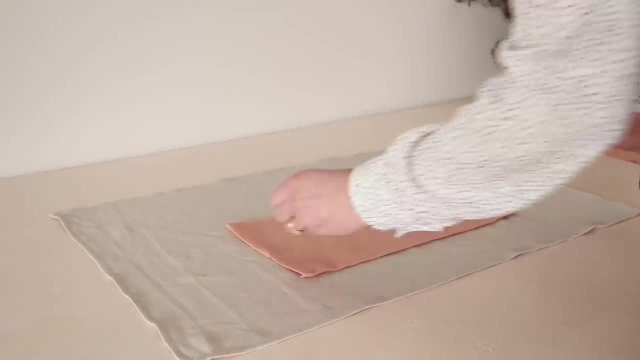 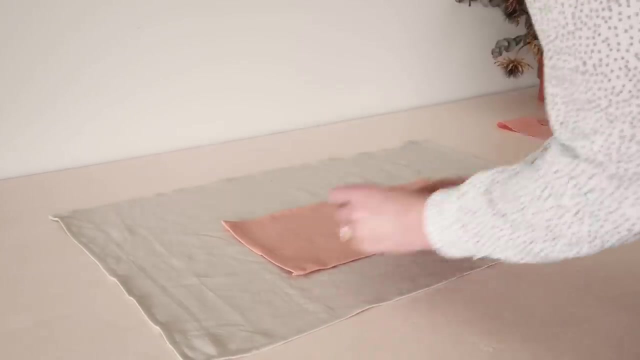 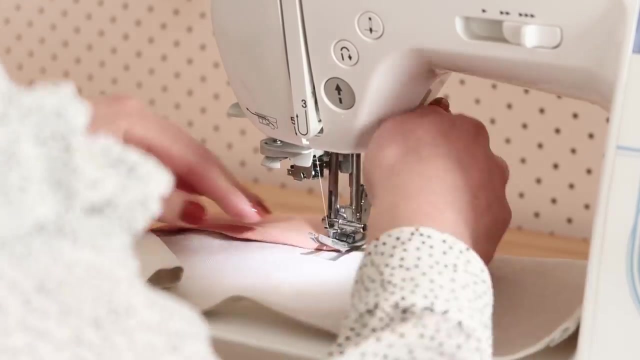 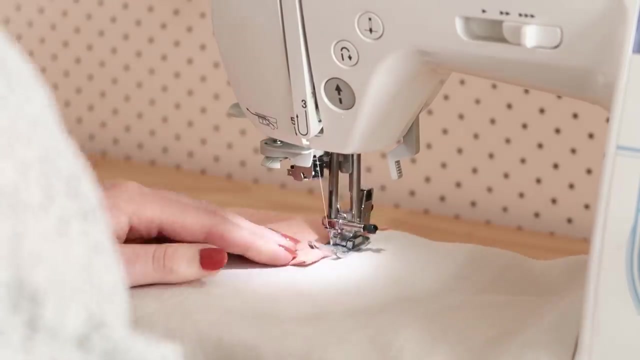 place the pocket onto the front of the apron, approximately ten centimeters or four inches from the bottom edge of the apron. stitch the pocket in place, leaving the top edge of the pocket open. prerecorded, cute and nice orangeорт firme pockets for an enemy. severe need for a chocolate covered apron length. 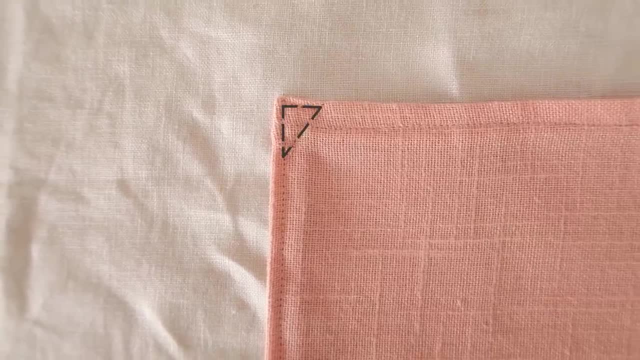 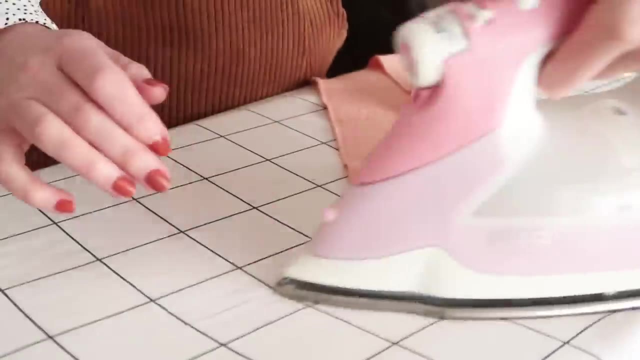 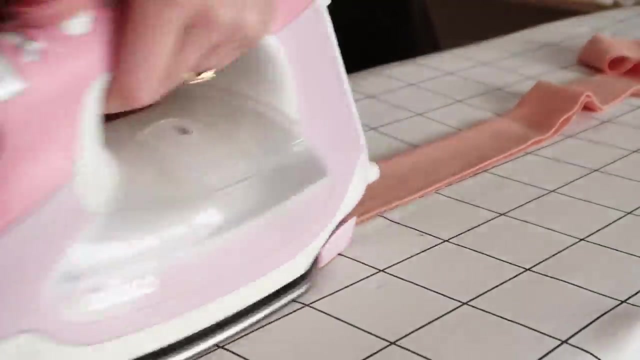 For extra strength. sew a triangle at the top of the pocket like this. Next, take the longer rectangles and fold and press the shorter edges in by one centimetre or half an inch, and then press the rectangles in half lengthways. Unfold the rectangle and then press the edges to the centre crease of the rectangle. 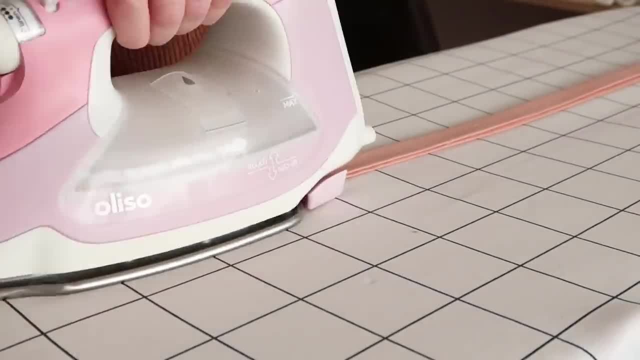 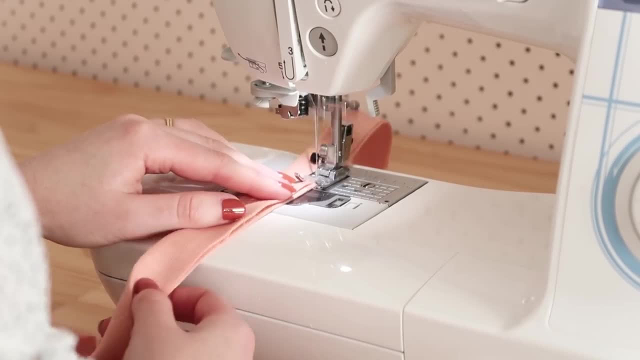 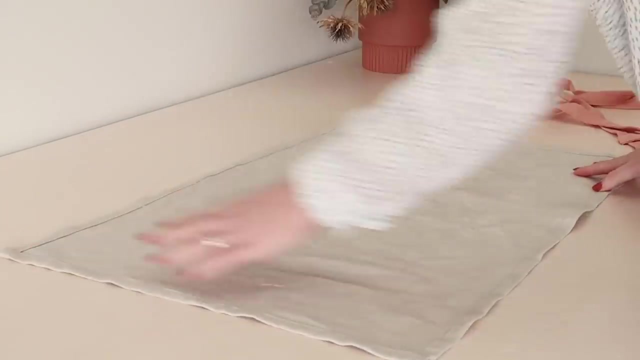 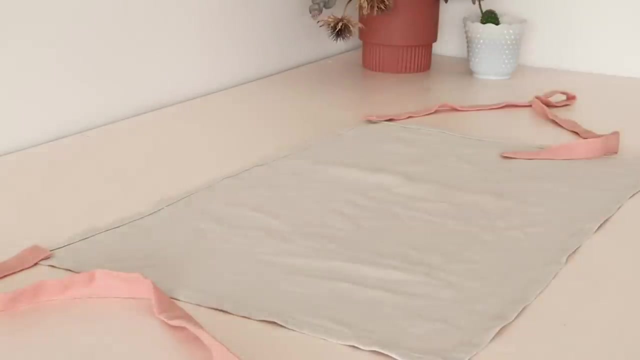 And then fold it in half once more. Stitch all of the folded edges in place. These will be the apron ties. Next, pin the ties to the back of the apron and then stitch them to the apron in a kind of circle. 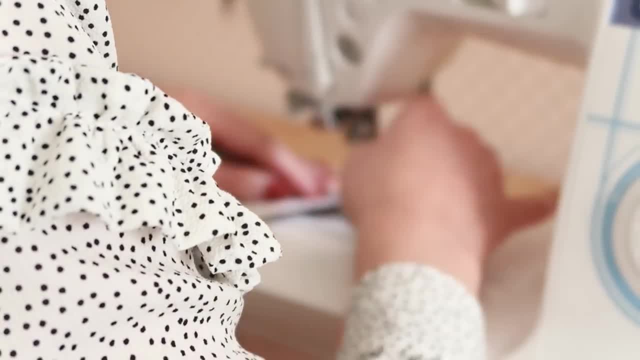 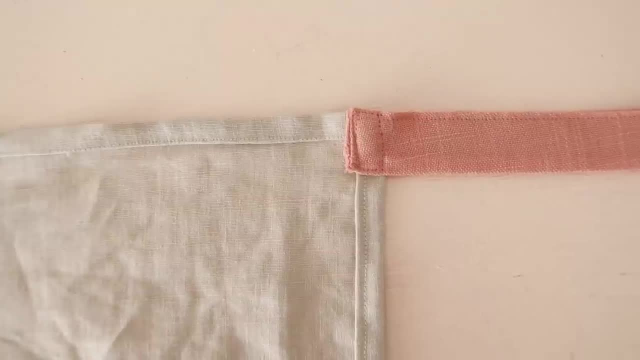 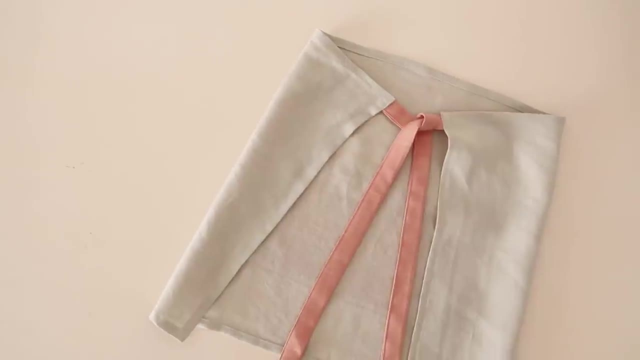 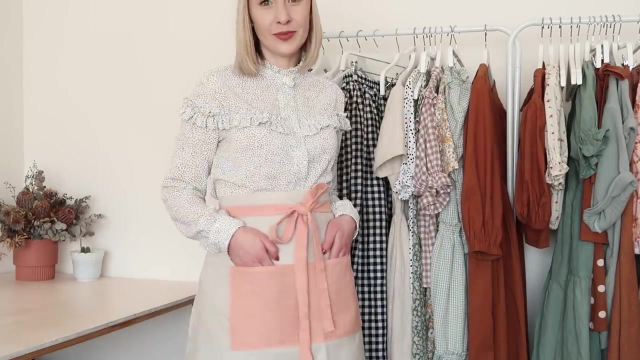 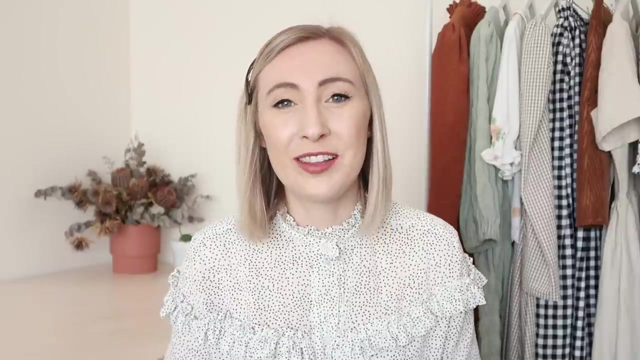 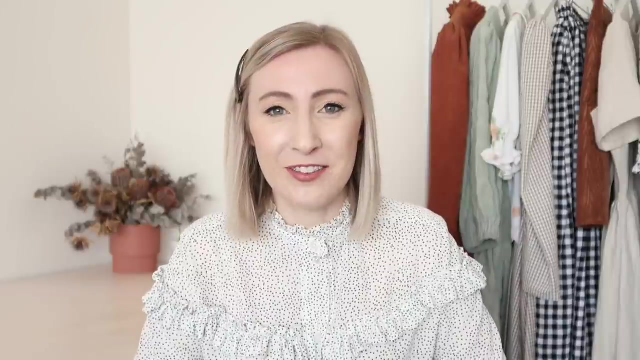 Like this And your super cute waist apron is complete. I hope you enjoyed this video and that it's given you some new ideas of some sewing projects to try. If you do have a go at any of the projects I've shared in this video, then I would love to see them. 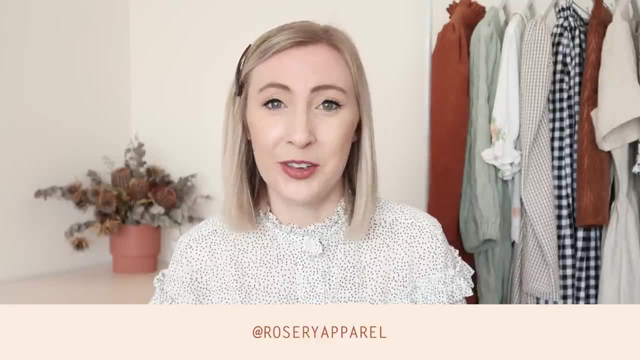 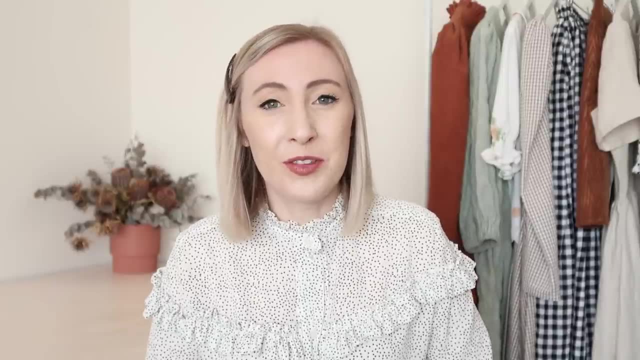 so be sure to tag me at Rosary Apparel when you share your photos on Instagram. And if you did enjoy the video, I would love it if you could give it a like and subscribe to this channel for more sewing type videos like this one. Have a lovely day and thanks for watching. 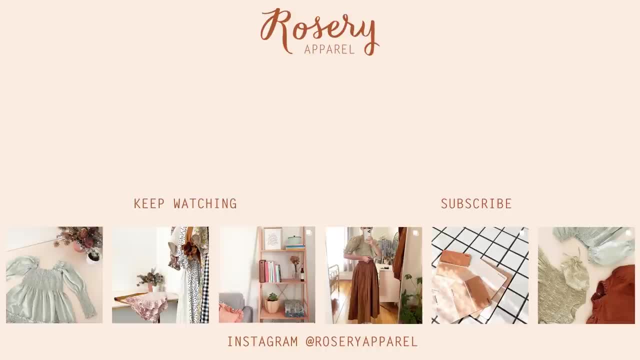 I'll see you in the next one.